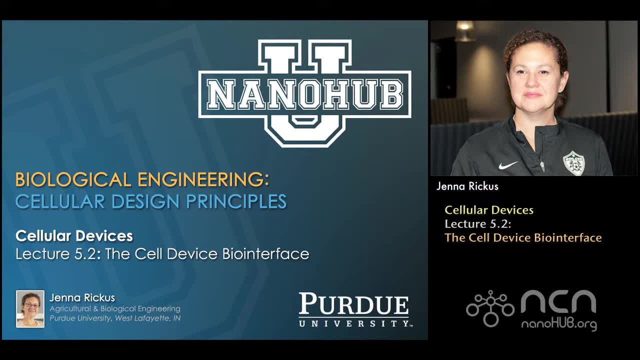 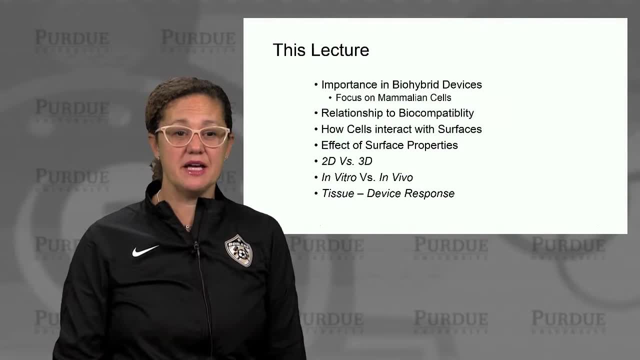 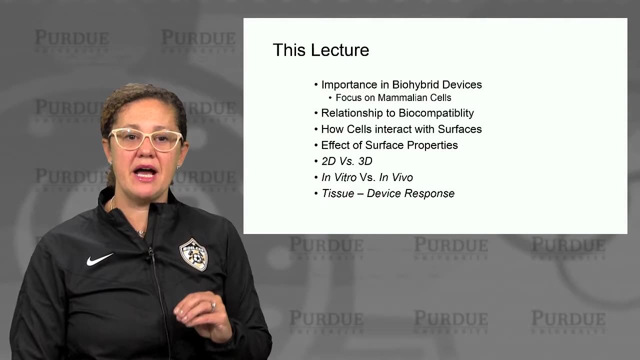 Welcome back. I'm Professor Rickus. In this lecture we're going to be talking about the cell-device biointerface. So first we're going to talk a little bit about the importance of this interface in biohybrid devices. 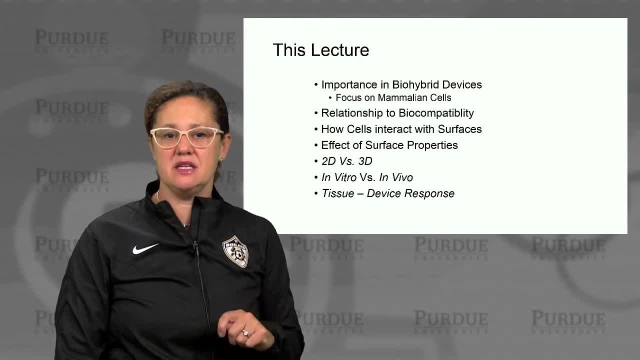 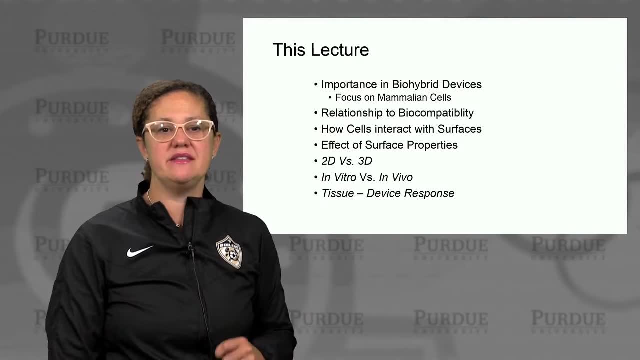 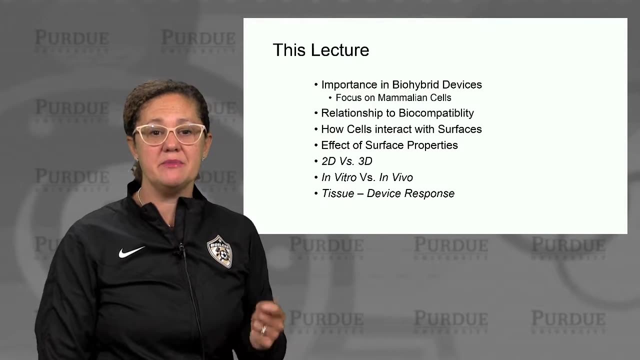 Our discussion today is going to focus primarily on mammalian cells and we'll return to bacteria and other prokaryotes later when we talk more broadly about cell-device integration. So we'll talk about the relationship of the cell-device biointerface to biocompatibility. 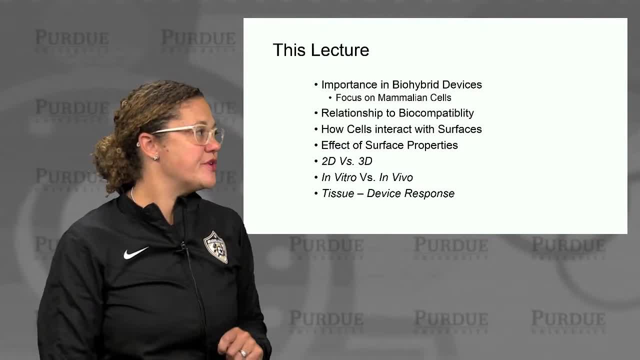 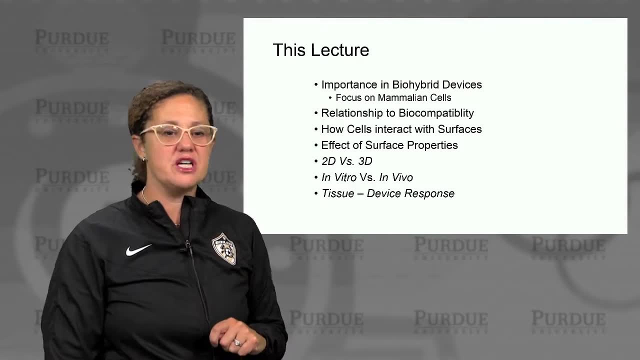 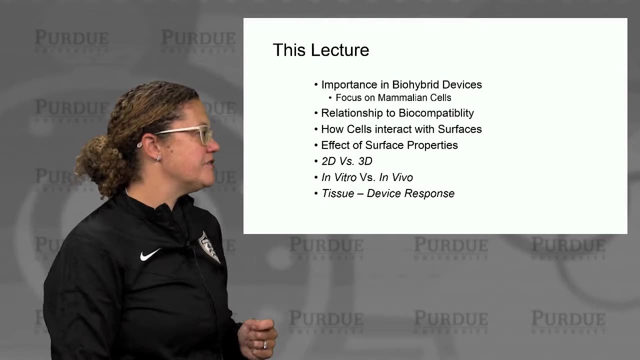 We'll talk about how cells interact with surfaces and the effect of different surface properties on cell adhesion and cell function. We'll highlight the difference between 2D integration and 3D integration and talk about some of the differences between an in vitro device and an in vivo device. 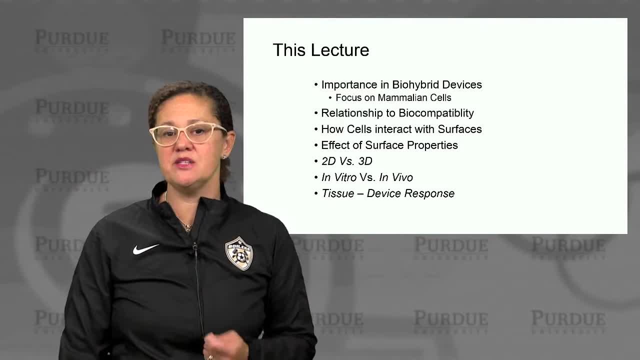 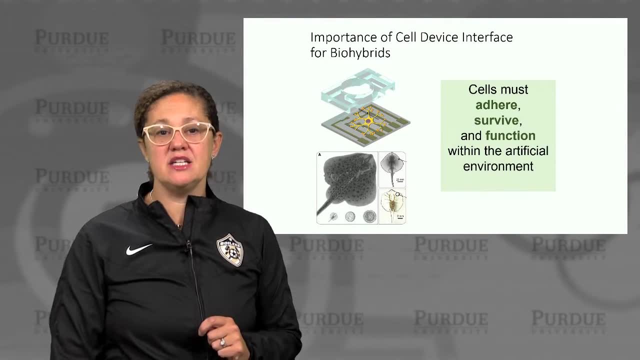 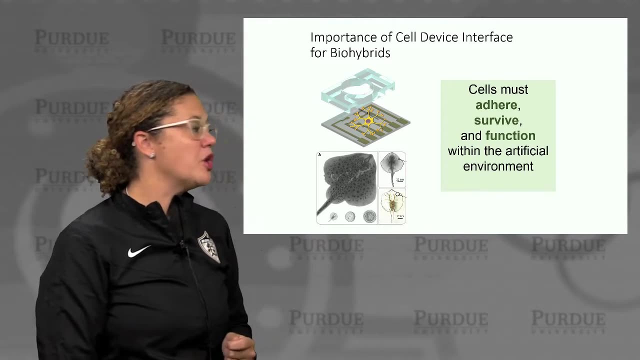 And that discussion will take place in a little bit. So let's take us into the tissue-device response for implanted devices. So, first thinking about the importance of the cell-device interface for biohybrid devices, In previous lecture we talked about this ray biohybrid robot that had living cardiac myocyte cells. 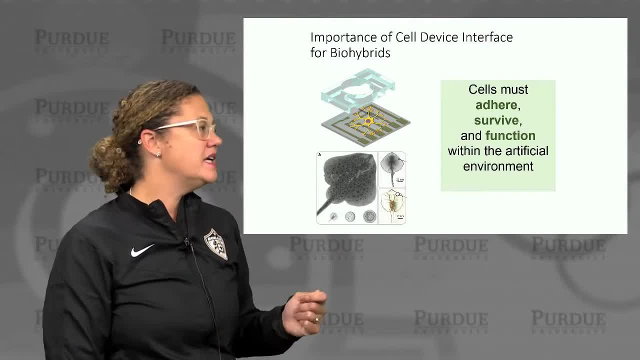 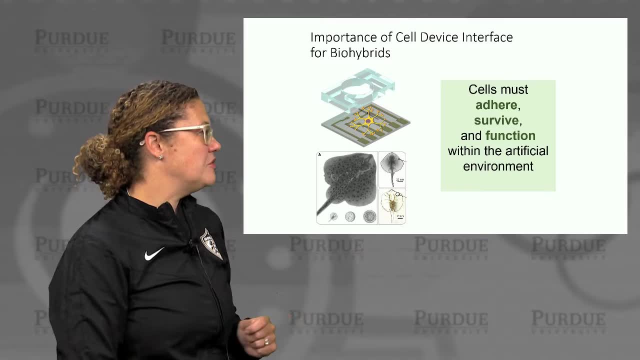 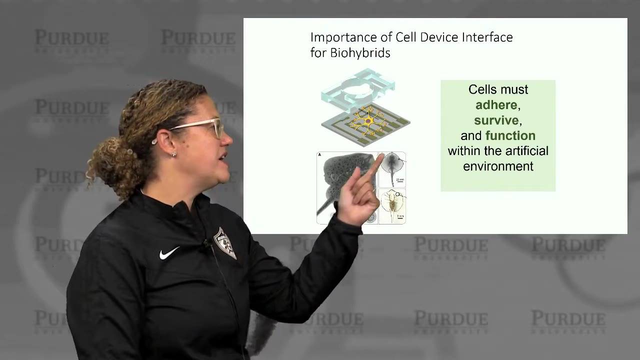 that formed essentially an artificial muscle in this metal and polymer-based robot system that could swim And if the cells rapidly thrived, it would Teethe up into our insides- or its inner- 1940s, in addition to being a fashion-loving protagonists. 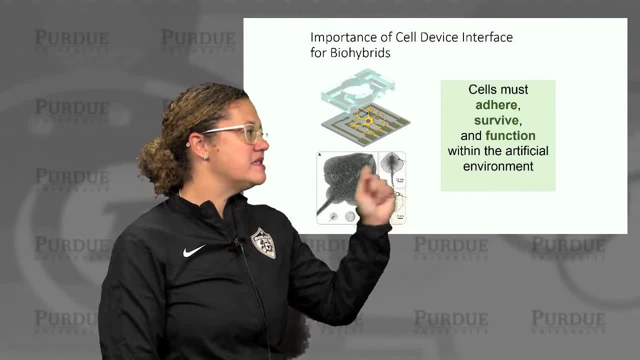 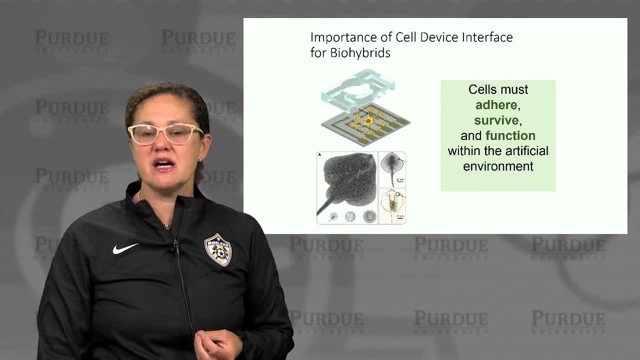 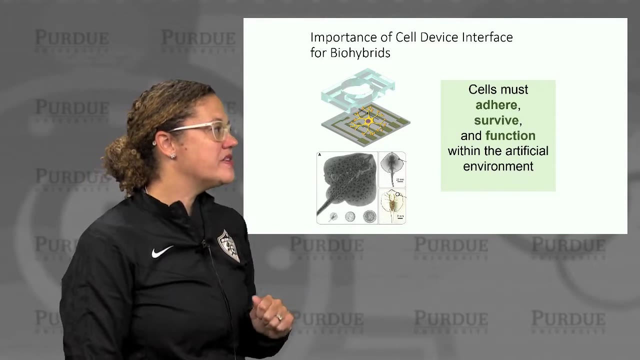 And then we also covered thisоз husky structure with germ thực, Which is 1 building a simultaneous serait, an initial emission. And then we talked about what this really was for the dropper: simply making sure this cell would treat it largelyformally. 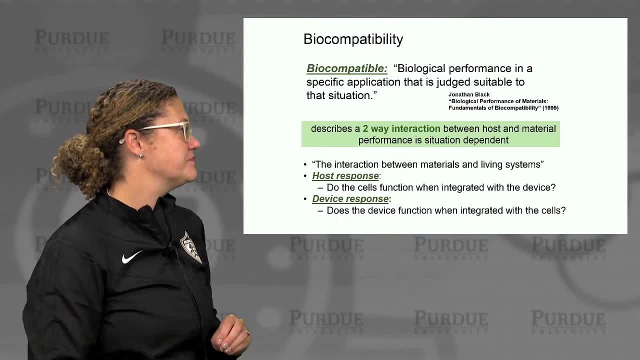 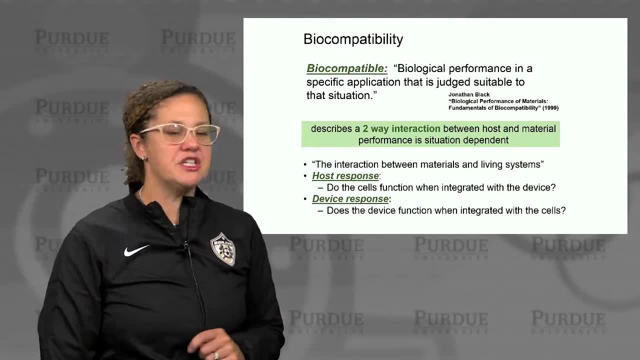 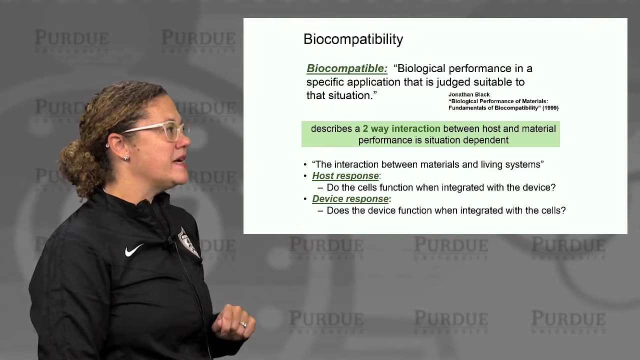 I just need to make this clear briefly. it affects survival and function happens Okay. so what's the relationship? You may have heard this word, biocompatibility- So here's a definition of biocompatibility that I favor. So biocompatibility will say something is biocompatible. 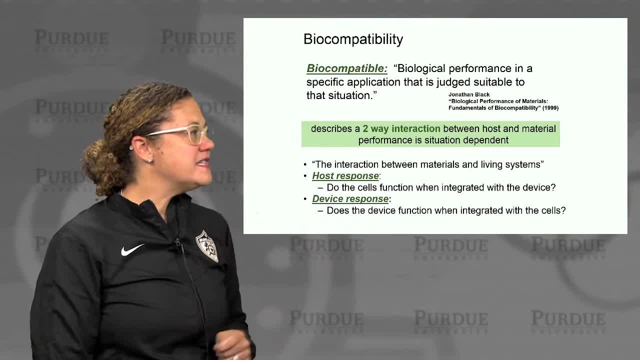 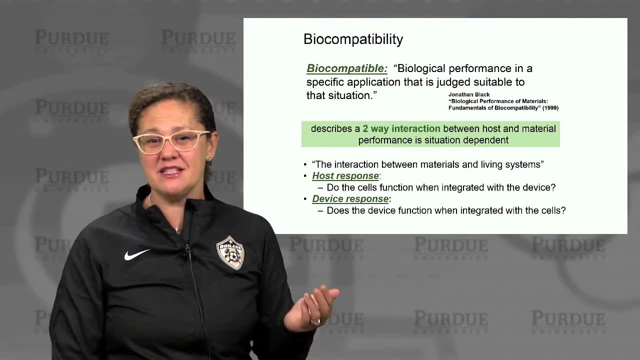 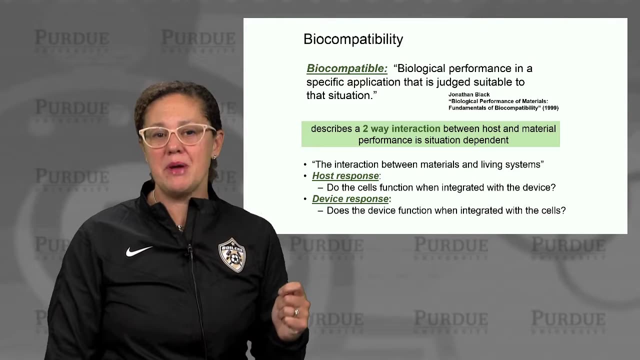 a biological performance in a specific application that is judged suitable to that situation. Now that seems somewhat vague and perhaps unsatisfactory to you, but let me tell you why I like this definition. If someone tells you that something is biocompatible, blanket biocompatible- 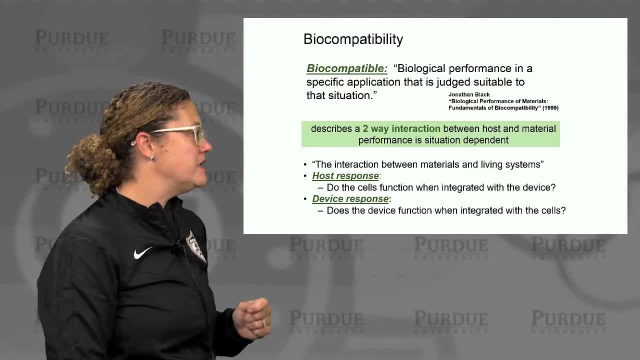 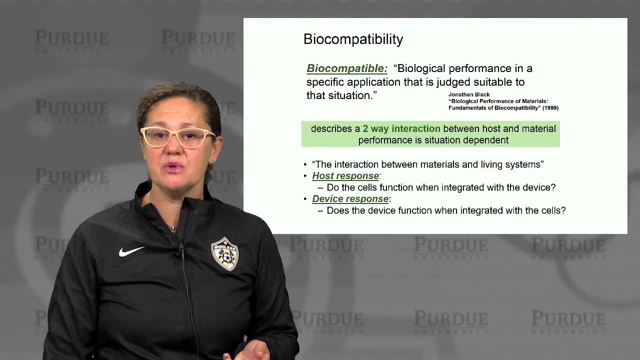 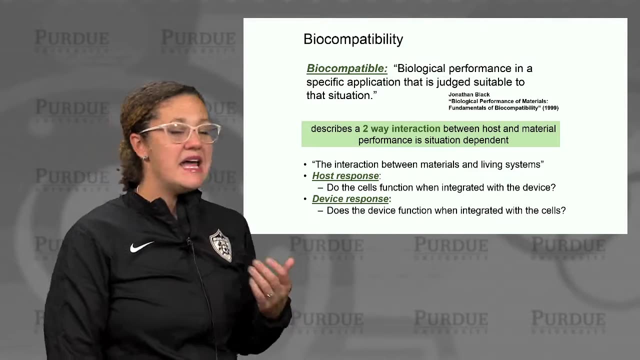 don't believe them. there's no such thing. Biocompatibility describes a two way interaction between the host, that is, our living cells that we're interested in, and the material or device. okay, And so the performance of both the cells and 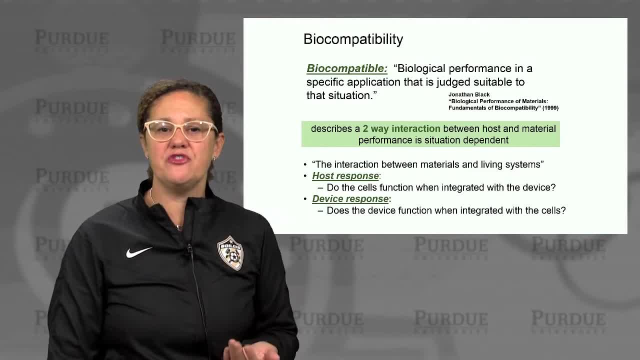 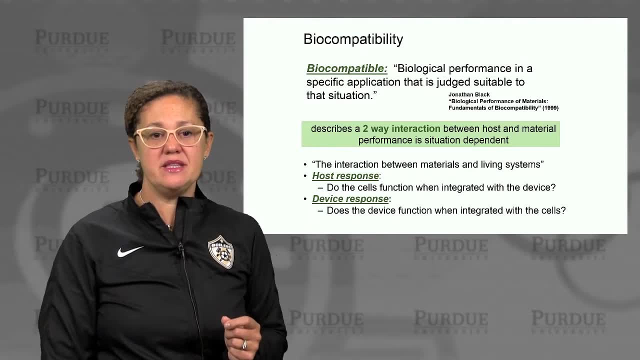 the performance of the biological system and material and device. what we measure as important, function or performance- is situation dependent, right, And there is always a two-way interaction between these things. So there is a host response. in other words, do the cells function? 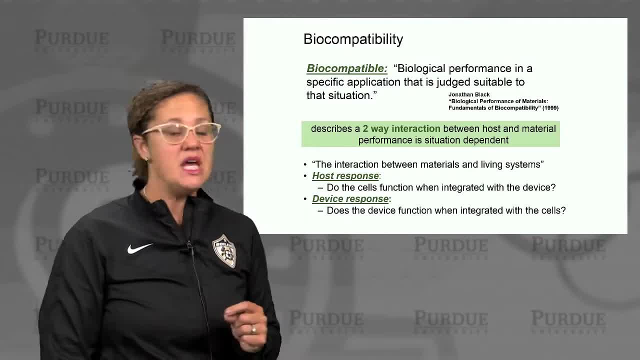 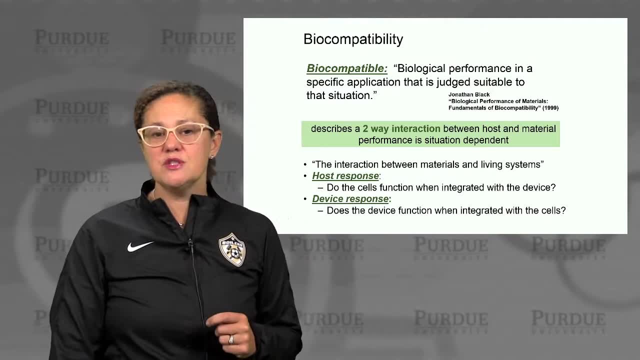 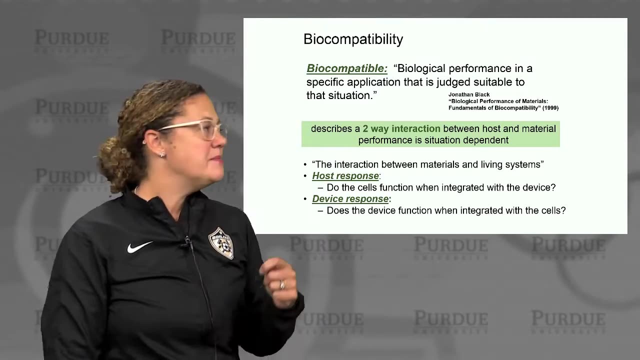 the way we want them to. when they're integrated with the device- And there's always a device response- Does the device function when integrated with the cells? So notice what's not in this definition. There's nothing about being inert or no interaction. 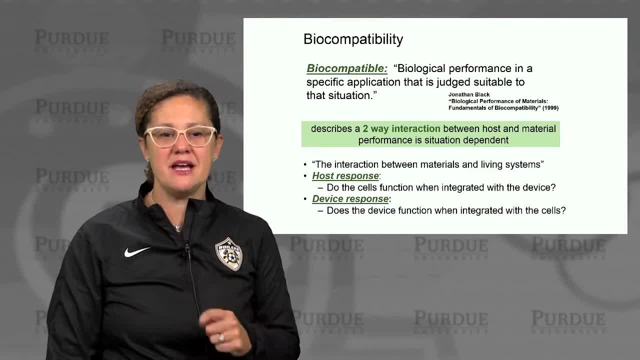 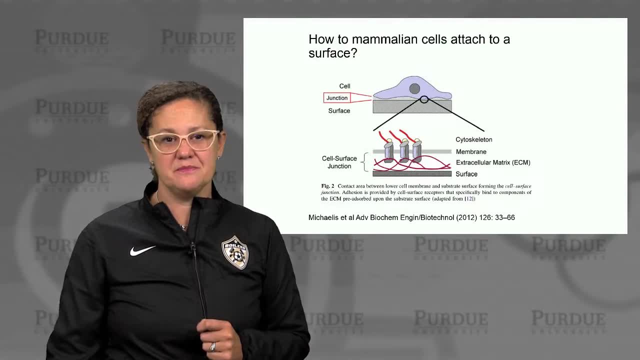 because that almost nearly never occurs. There's almost always some interaction, And the question is: is it an interaction that we want and is beneficial to our bio-hybrid device? Okay, so let's talk about these interactions a little bit more specifically. 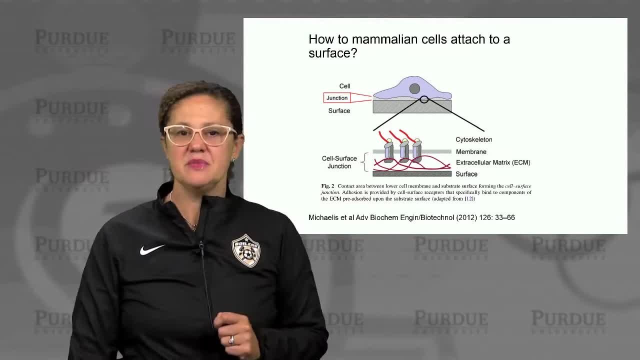 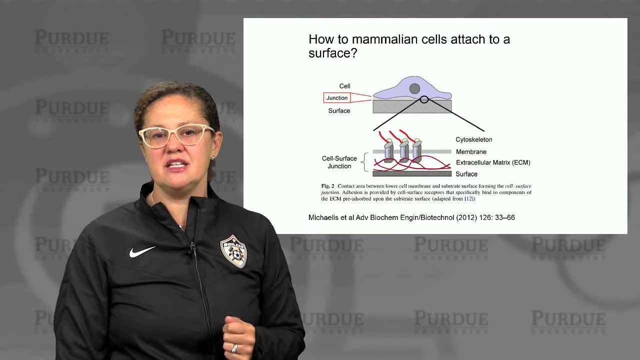 How do mammalian cells attach to a surface? So here in the top we have sort of a zoomed out view, thinking about the cell And this is the surface of our device that it's interacting with. And if we focus in on this junction area now and 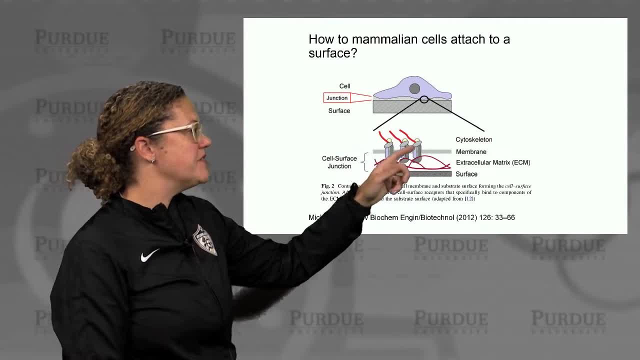 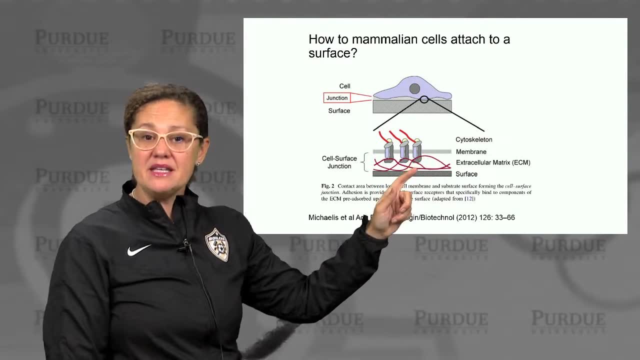 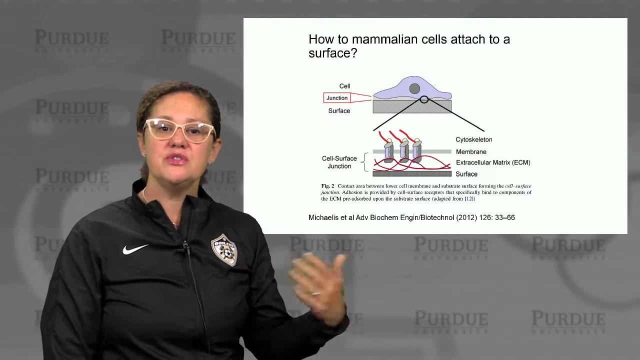 think about what's really happening. So here we've got a zoom in of the cell membrane. Remember, cell membranes have proteins that are embedded in these membranes, that act as their receptors and they really relay information from the outside of the cell to the inside of the cell, both through cytoskeletal components and 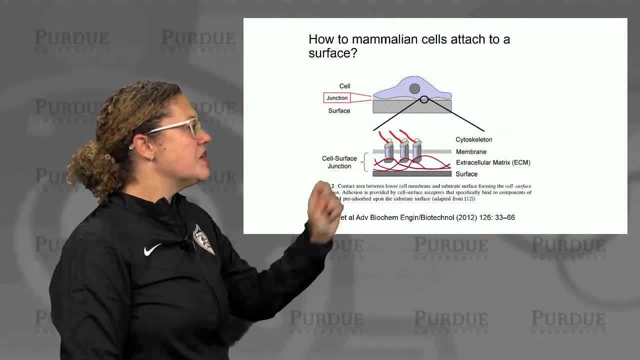 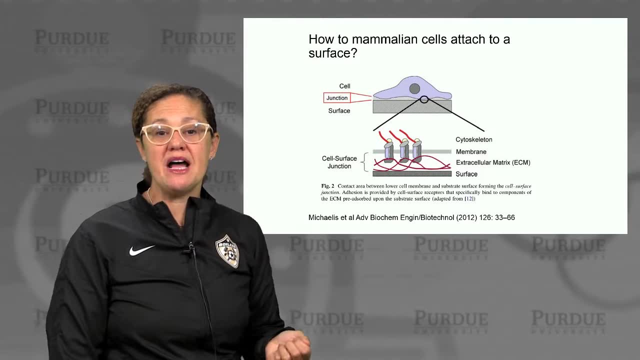 through soluble. So how does the cell really attach to the surface? Well, there are extracellular proteins, often produced by the cells themselves, that are laid down, and it's these extracellular proteins that act as adapters. They bind to receptors on the cell membrane and 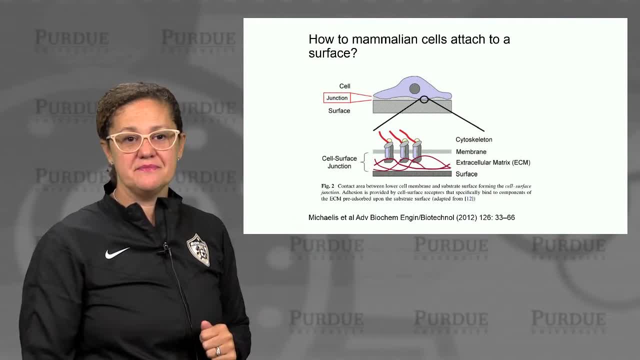 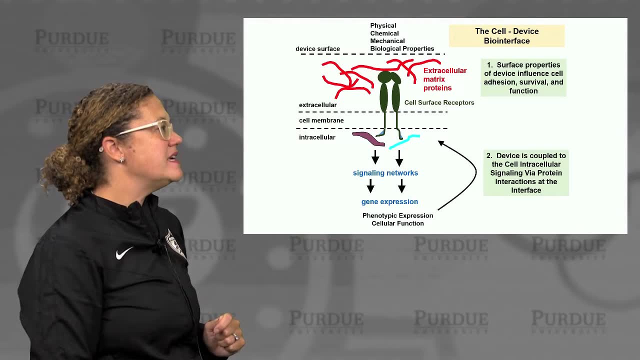 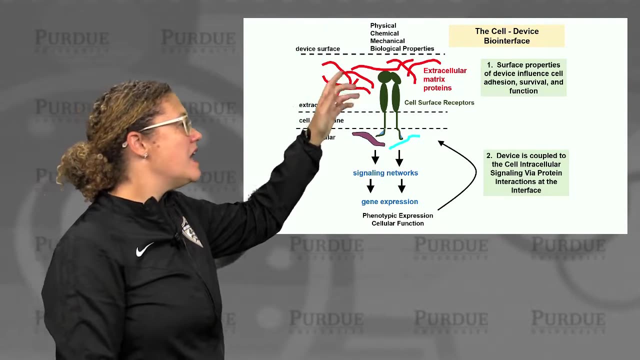 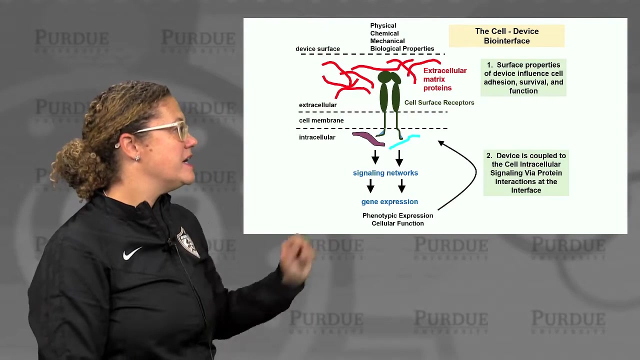 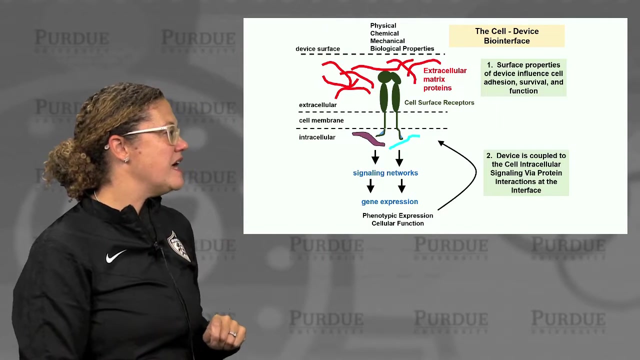 they adhere and interact with the surface. So in this way, thinking a little bit more directly about the cell device interface, we can see that the physical, chemical, mechanical properties and biological properties of our device surface influence our cell function downstream by interacting with extracellular proteins that interact with receptors on the cell. 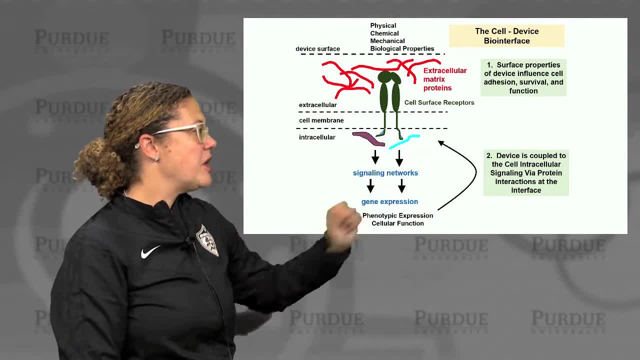 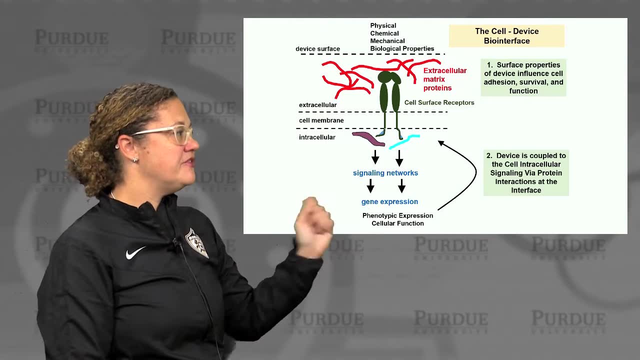 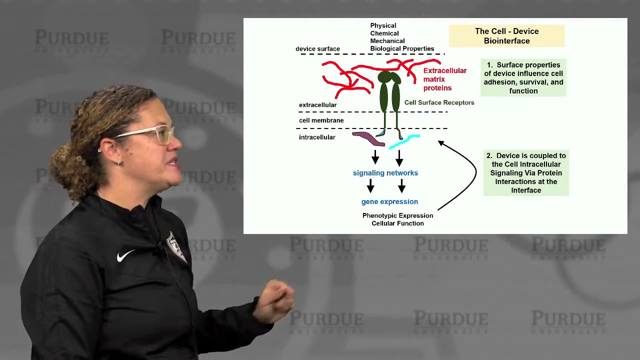 that relay that information to the intracellular part of the cell, including the cytoskeleton. So we can see that the cell's intracellular signaling and other components of signaling networks that can ultimately affect gene expression and the phenotype or function of our cells. 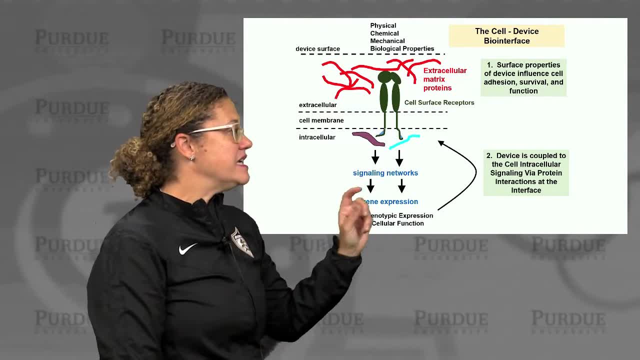 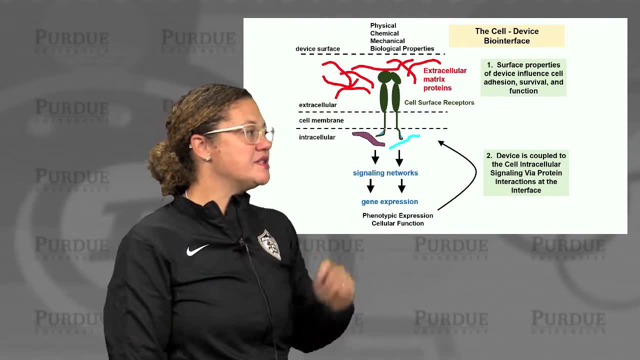 So there's two key points here: One, that the surface properties of our device influence directly the cell adhesion, survival and function, and that the device is really directly coupled to the cell's intracellular signaling via protein interactions at the interface. 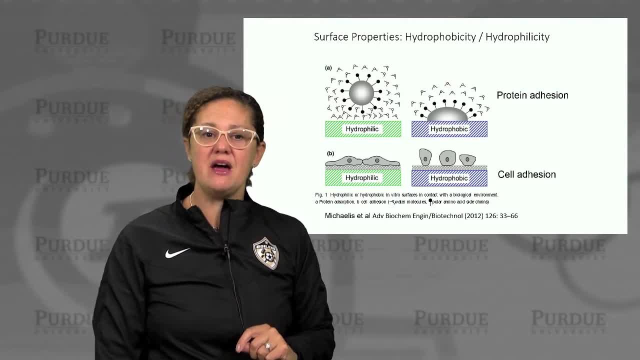 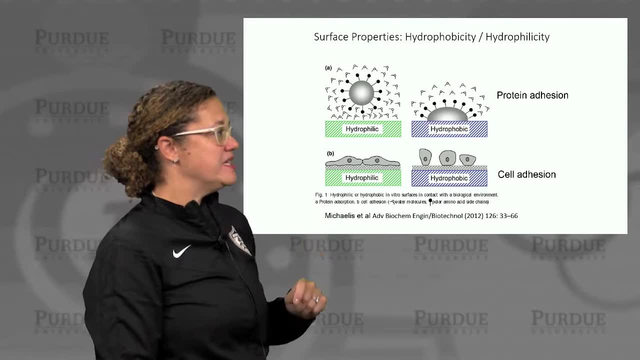 So this gives us a framework to dig in a little bit more deeply and we can think about how do surface properties affect cell attachment? Well, one of the most basic surface properties is the hydrophobicity or hydrophilicity of the cell's surface. 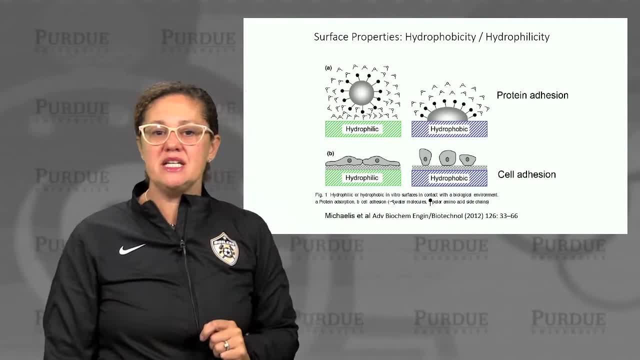 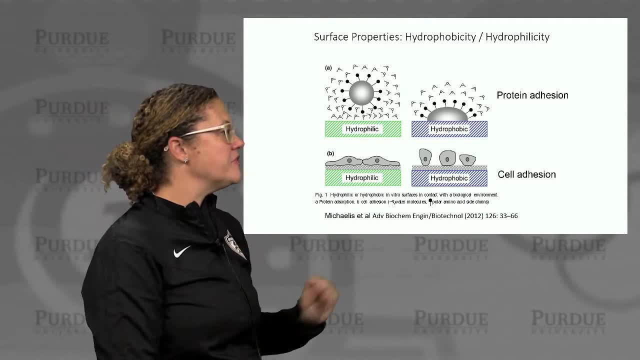 And this will affect both the directly, the protein adhesion, including those proteins that cells use to attach to, to adhere, And we can also think about it from a more zoomed out view- and how those cells will, how they will spread out. 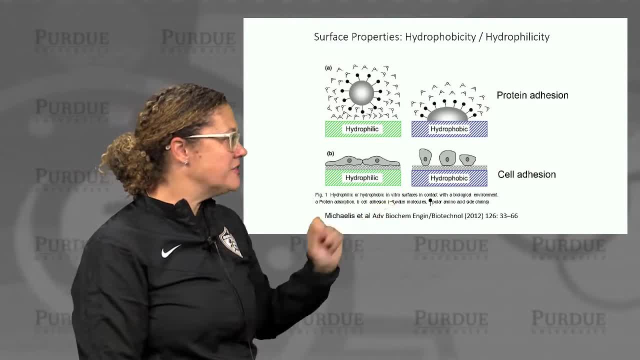 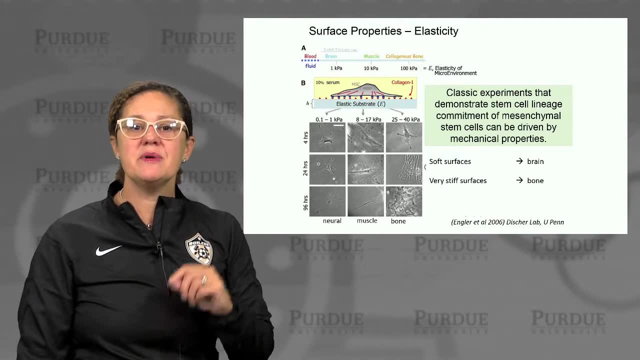 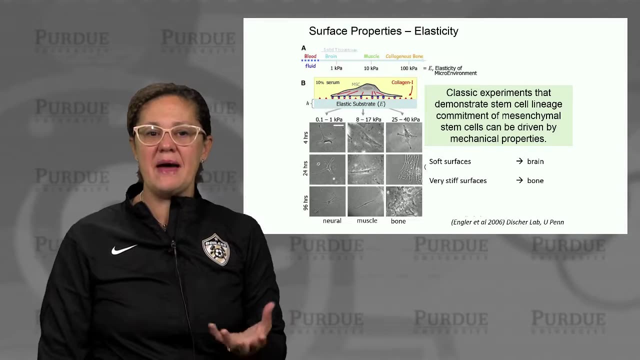 And lay down on the surface in a hydrophilic state versus a hydrophobic state. Another very important property of the surface are the mechanical properties. One of those properties that's been looked at extensively is elasticity, the elasticity of that matrix. Essentially thinking, you'd think about how stiff or 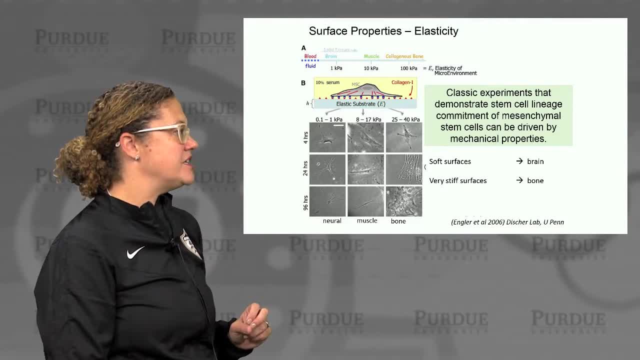 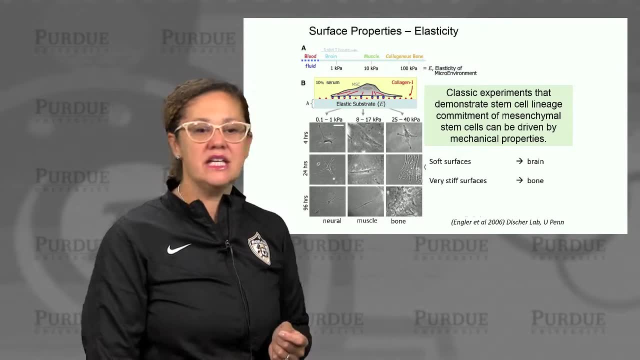 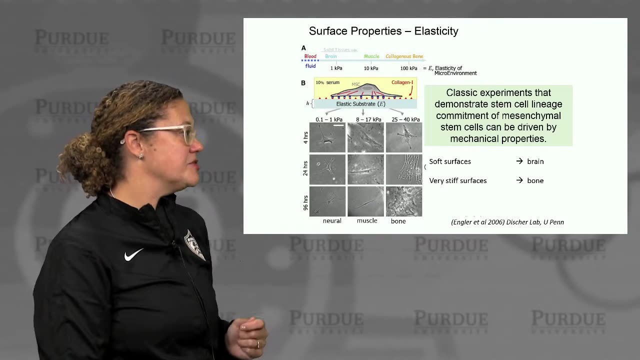 how elastic that material is that the cells are attaching to, And here's some data from some now classic experiments That demonstrated that even the stem cell lineage commitment- So in other words, what type of cell a stem cell turns into right for these mesenchymal stem cells- can be driven by mechanical properties. 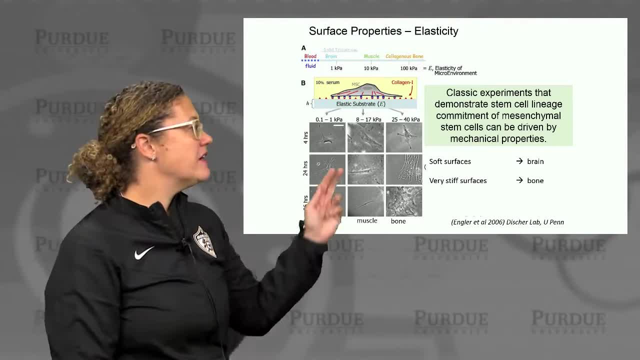 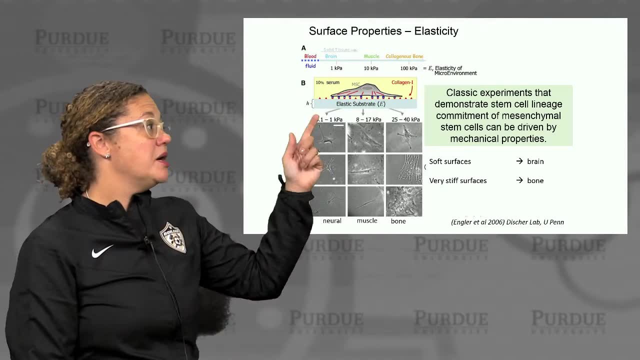 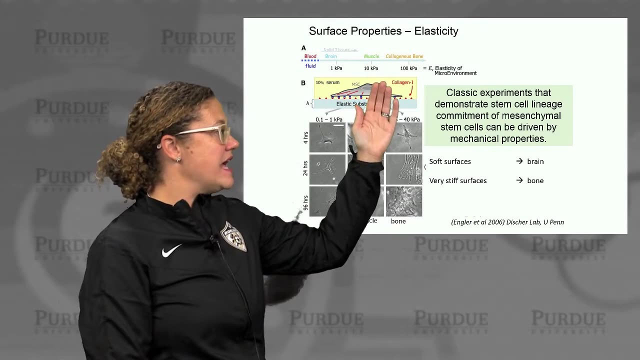 So these same cells in the same environment, varying only the stiffness of the substrate. you can induce these cells to differentiate into brain-like neural cells. if they're on very soft materials, Right, And as that material gets more stiff then you can induce them to differentiate. 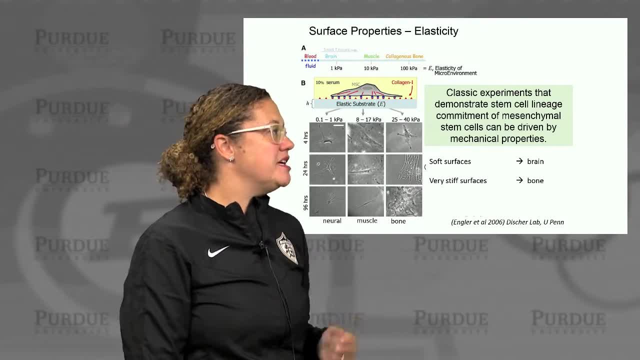 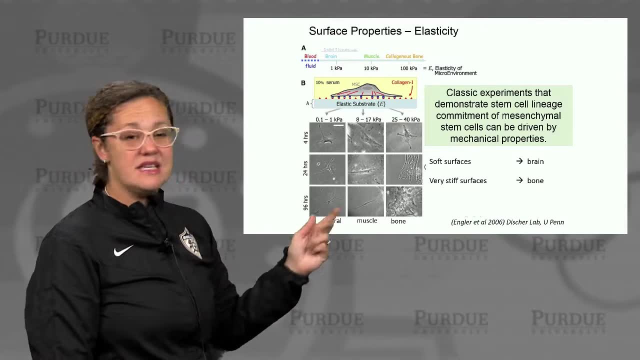 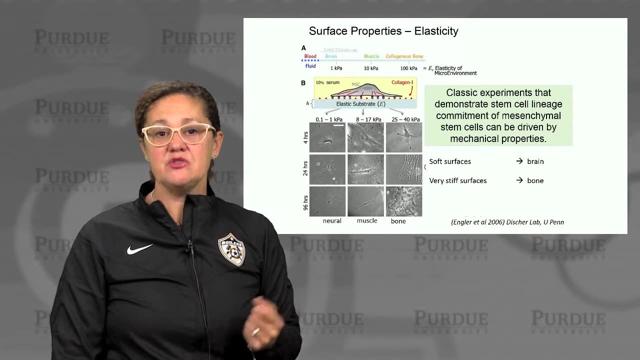 into muscle or, at the most stiff material, you can induce them to differentiate into bone-like cells, right. So this is, as I said, a classic example, and a dramatic one, that shows how the mechanical properties of the surface can dramatically influence cell fate, and 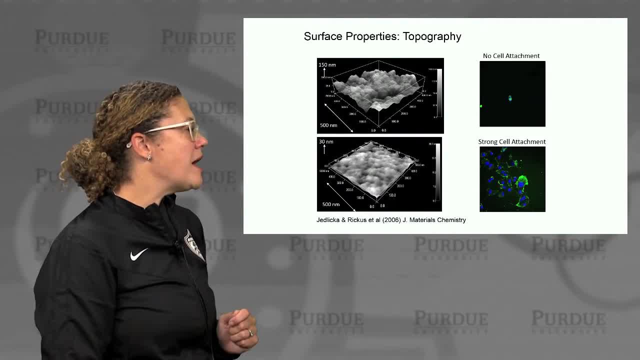 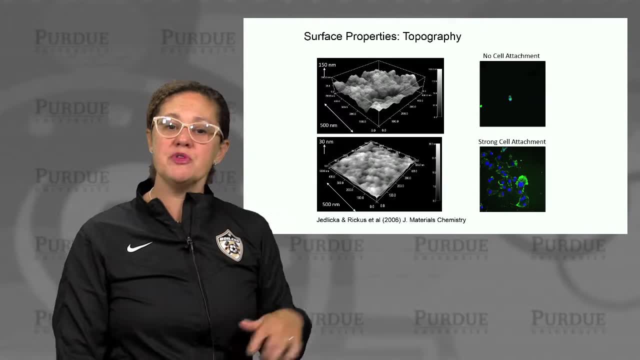 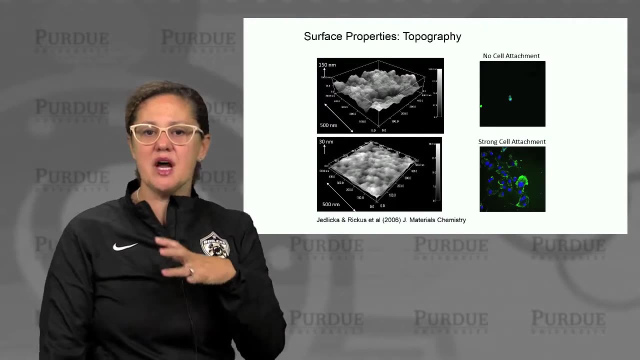 their function. So another property that can be very important is the topography, particularly at the nano and the microscale. Remember these proteins that are adhering. Proteins adhere really, they're living in the nanoscale right And cells are microscale structures. 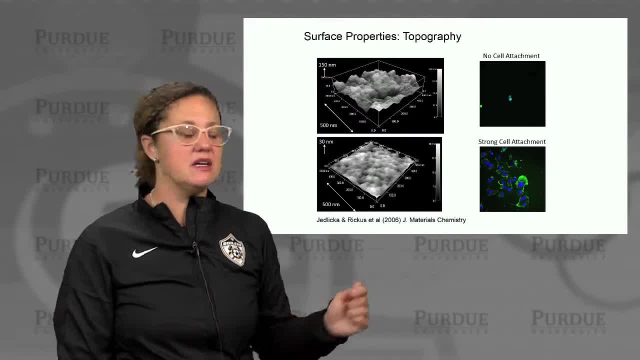 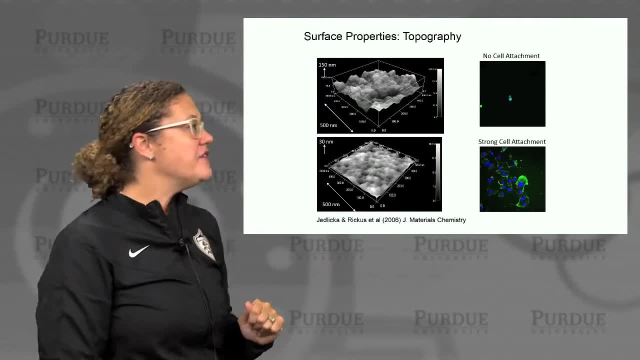 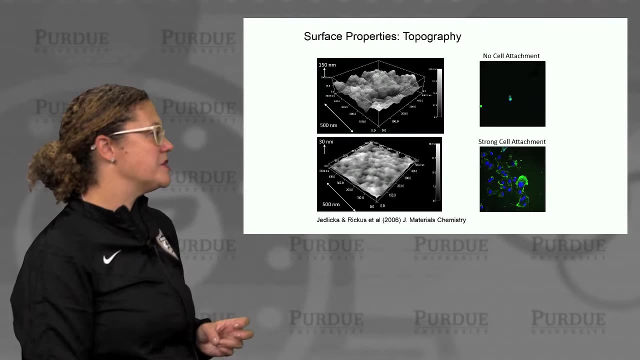 So here we have two materials. These are silica-based materials produced in my lab. They are identical chemically in every way. They've only been processed differently in order to change their surface topography. And so here we see an atomic force microscope image of these two materials. 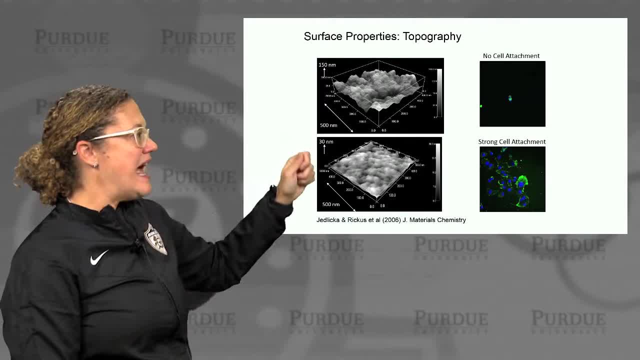 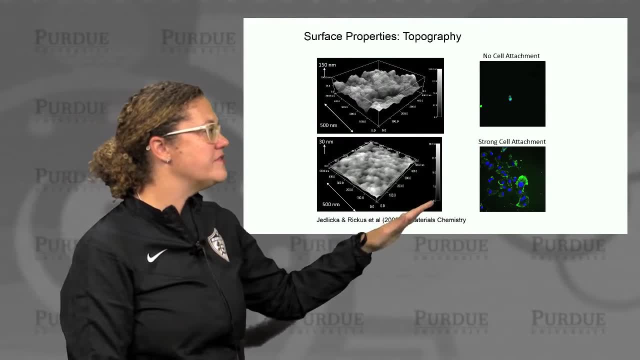 one that's very rough on the nanoscale. And notice these axes even are different. So this axis here is about 150 nanometers, whereas this you can see, this material is very, very smooth, Sub 30 nanometer surface features on this material. 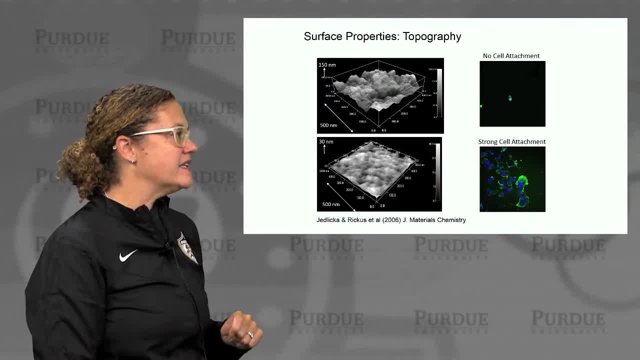 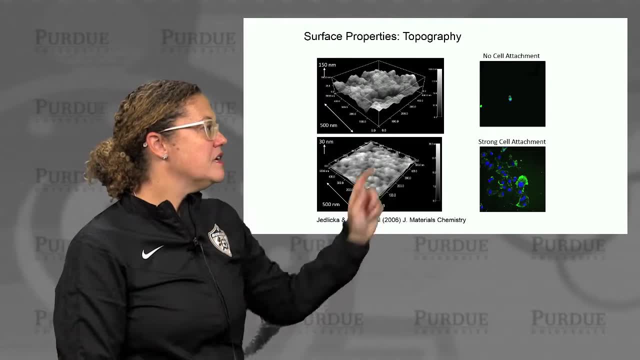 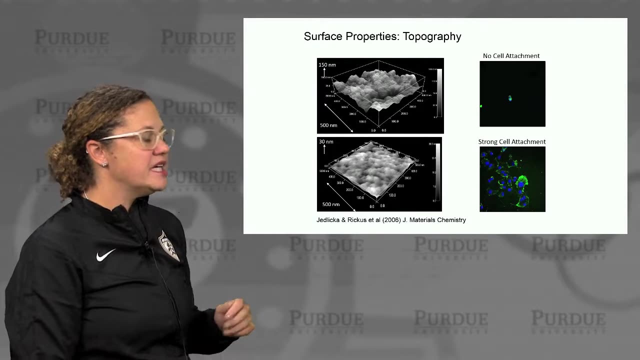 And just by changing the surface topography we can dramatically affect how neural cells attach to this surface. So on the nanoscale rough material, we see almost no neural attachment to these surfaces, While the same material of identical chemistry, now that's much smoother on. 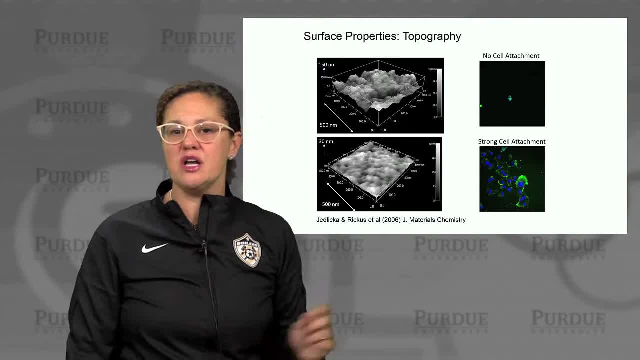 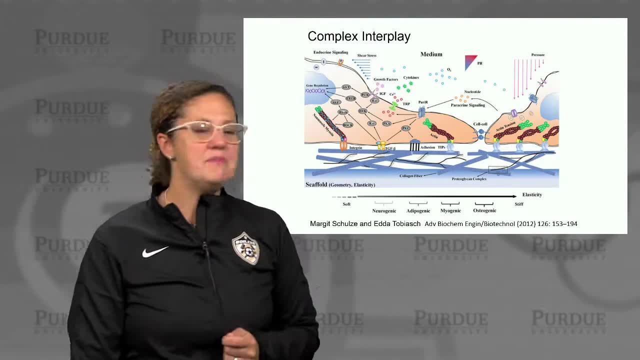 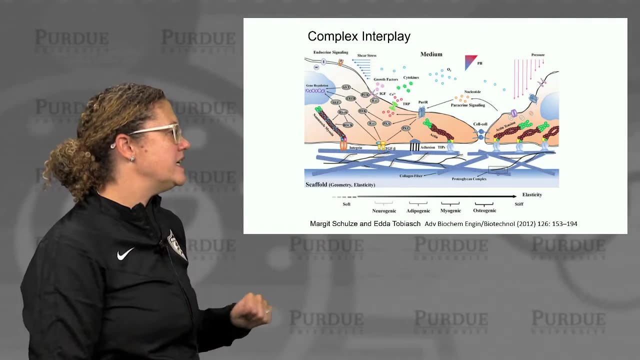 this size scale we can get very strong and nice neural cell attachment to these surfaces. So I put this figure up just to show you and sort of put in your mind the complexity of this interplay. Again, we're looking at from this surface or scaffold. 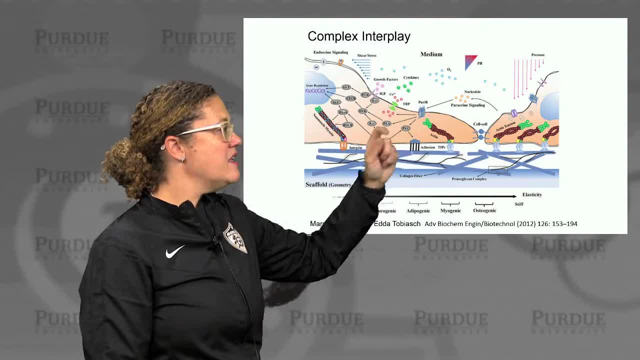 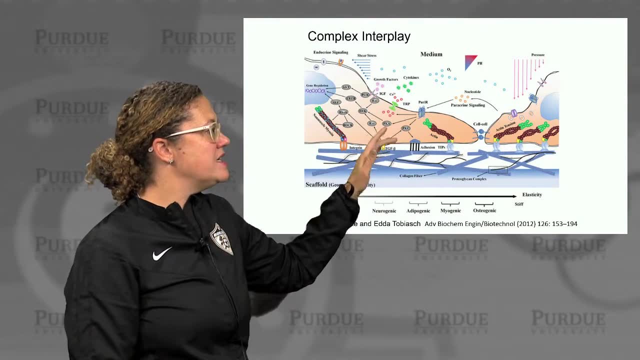 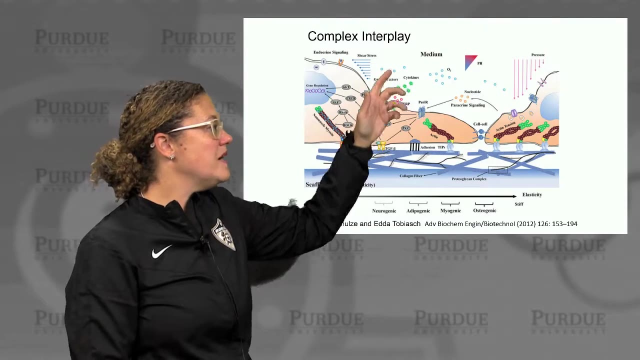 interacting through these protein layers with the cell versus multiple different types of receptors and adhesion molecules, coupling into both the cytoskeletal elements as well as the complex signaling network of the cell, and, as well, interacting with the soluble and interstitial volume in space and 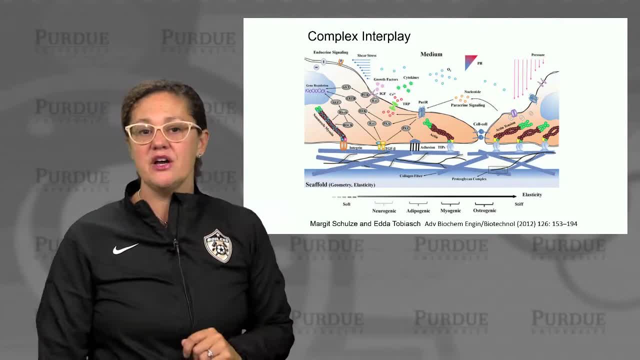 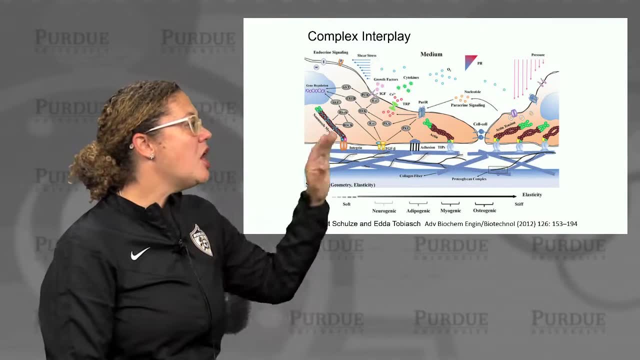 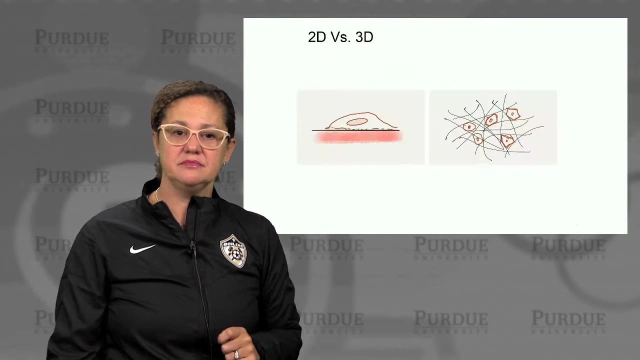 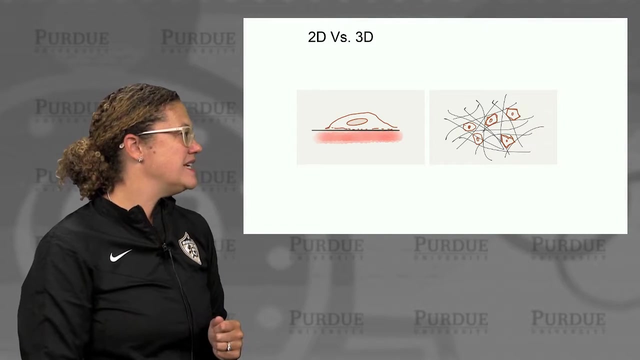 the signaling that's happening in here, as well as any other physical inputs such as pressure and shear force from, for example, fluid flow. So all of these things are interacting to influence how those cells adhere, survive and function. Okay, so we've mostly been talking about cell biointerface in a 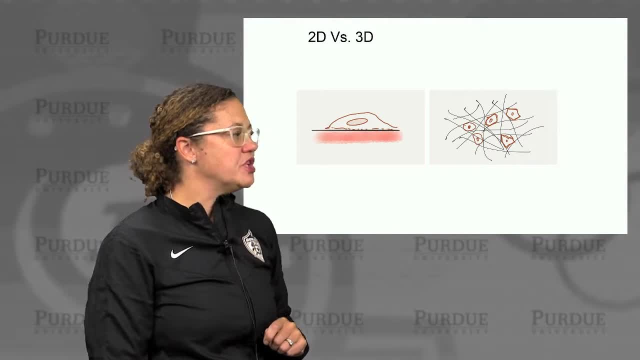 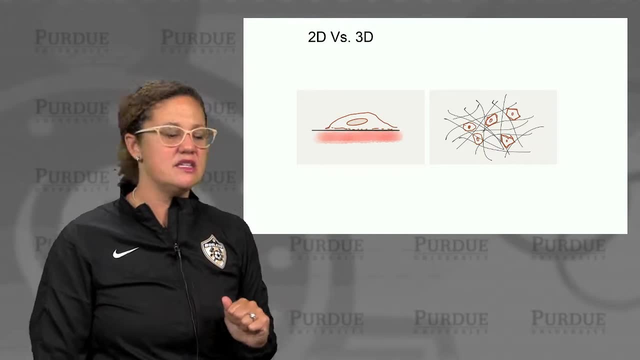 two-dimensional context, But quite often we're also looking at cells in a three-dimensional context, And so I put up this cartoon here that I made as sort of articulate these two things: one, looking at the cell attaching to a planar surface. 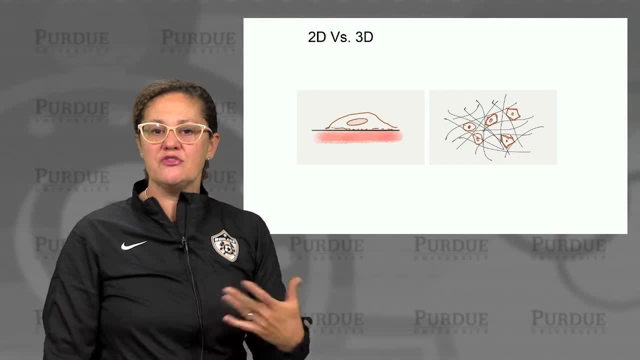 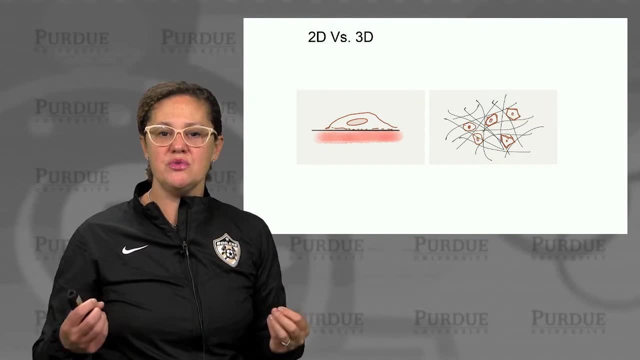 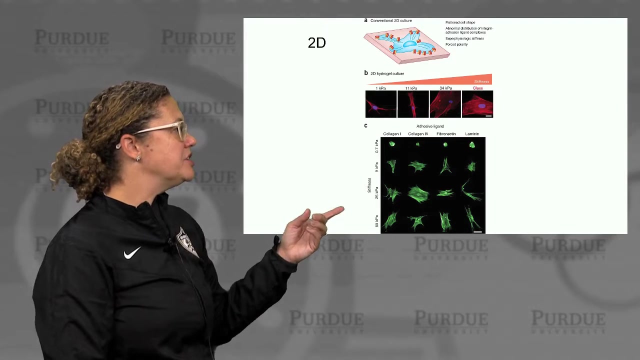 versus cells that may be within a matrix, artificial that may be integrated into a device And you can see how they're interacting with and adhering to the artificial components Are- Can be very different. So in a two-dimensional we typically get a very flattened cell shape and 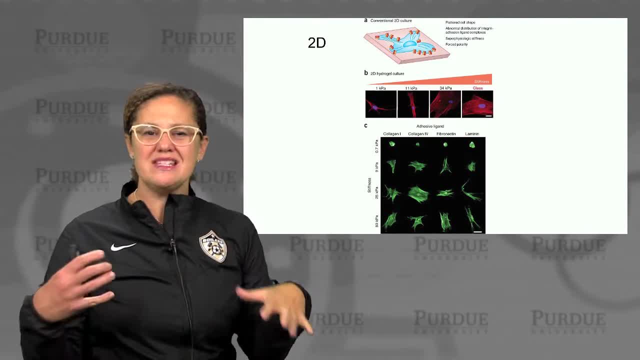 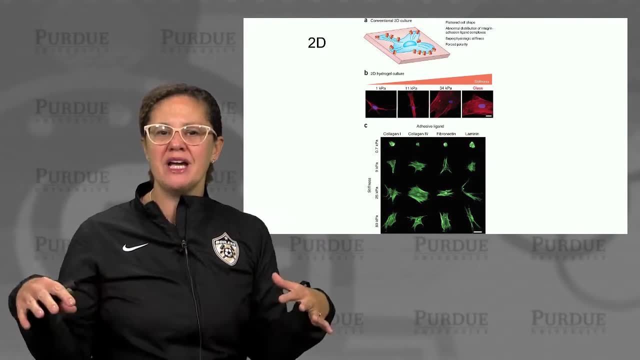 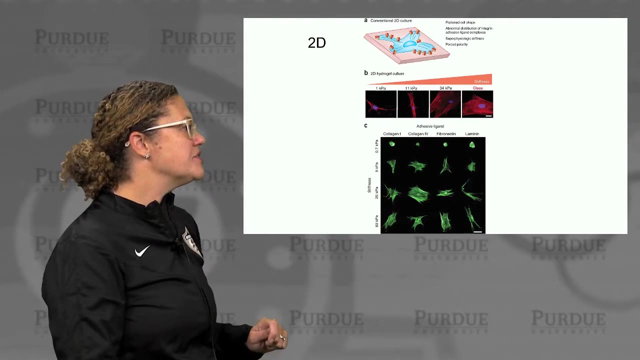 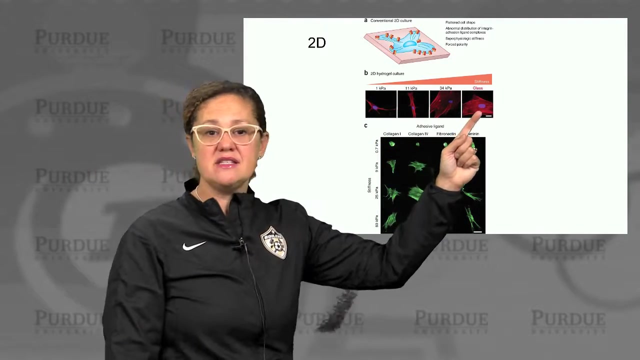 actually an abnormal distribution of these receptor adhesion ligand complexes. So there's often this forced polarity and abnormal morphology in this sort of planar orientation And cells are very dramatically- again you can see how their morphology even changes Again, as we vary stiffness, as we looked at before. 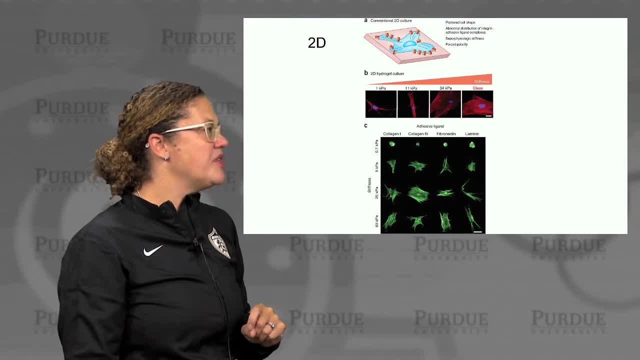 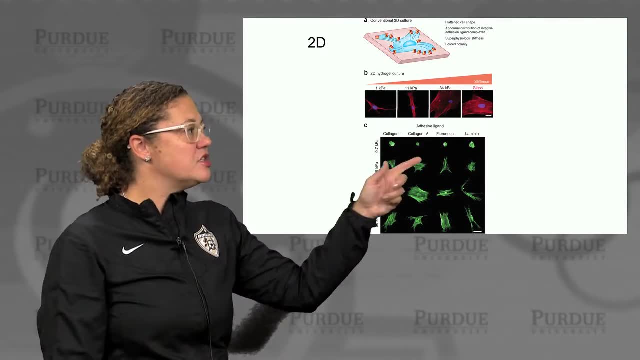 So now you're sort of seeing the attachment points and how the cells sort of spread out and have these different morphological shapes which you can imagine has a direct impact on the signaling and how they're functioning and what's happening internally to the cells. 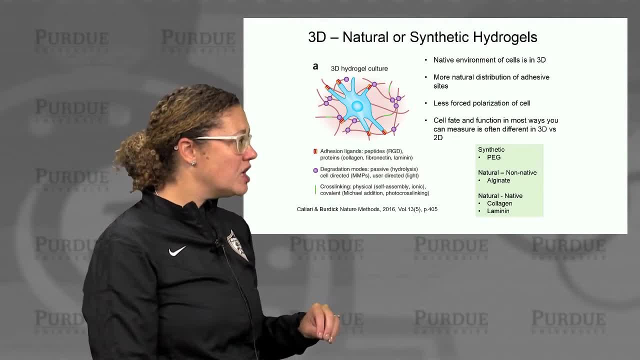 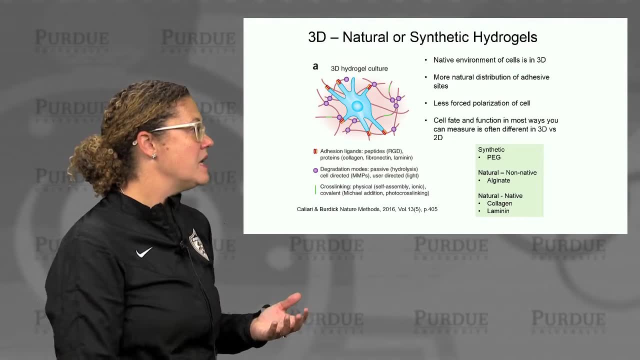 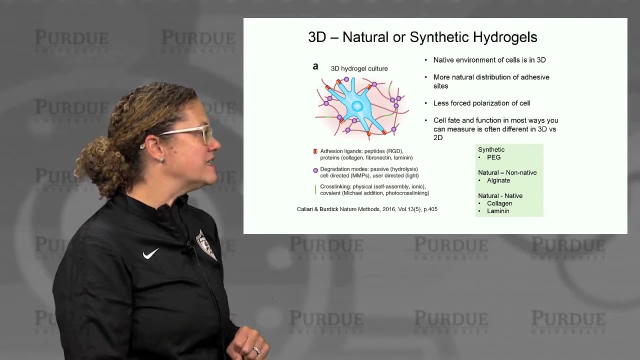 Whereas 3D is generally considered a bit more of a native environment. This is how cells tip, Typically live in a three-dimensional sorts of environment, And so they often have a more natural distribution of adhesive sites with the material that they're interacting with. 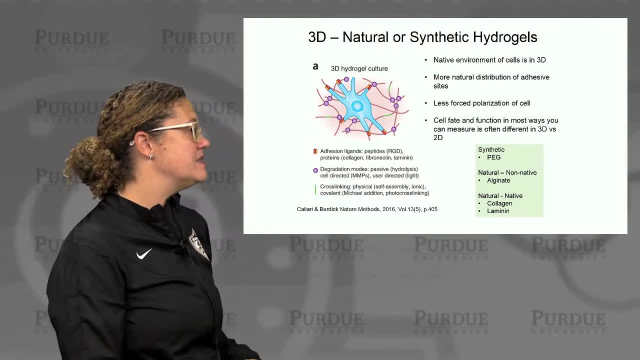 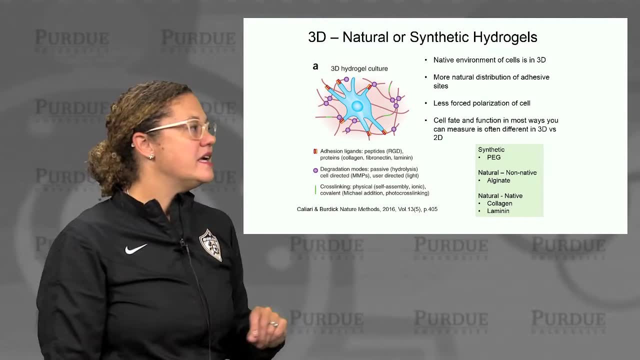 And less of a forced polarization state that can influence cell fate And in many ways this sort of cell fate and function, in most of the ways that you can measure, is often different for the same cell if you are to interface it in a three-dimensional environment. 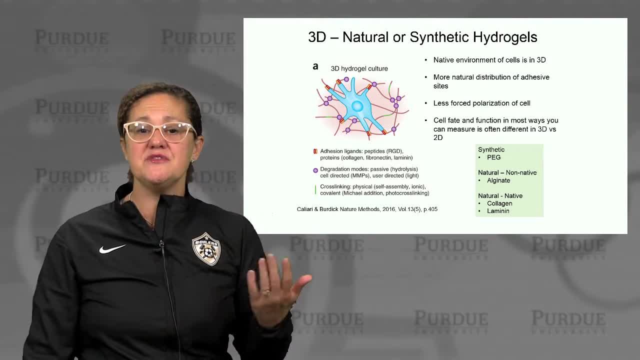 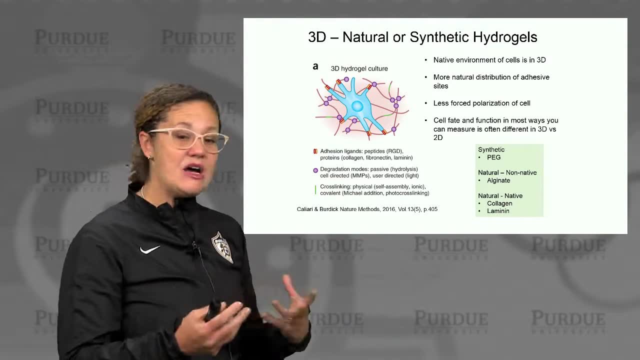 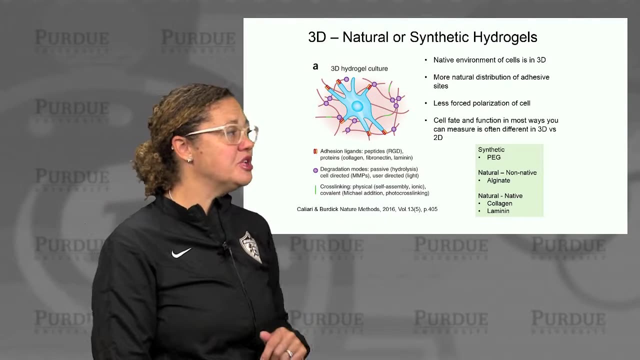 versus a 2D environment. Now, for the sake of devices. there are different types of three-dimensional materials that we often use to house cells and devices. They can be synthetic, such as a PEG-based system. It can be natural and non-native, such as alginate polymers. 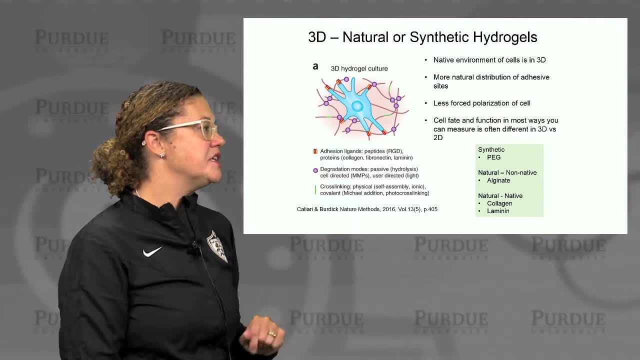 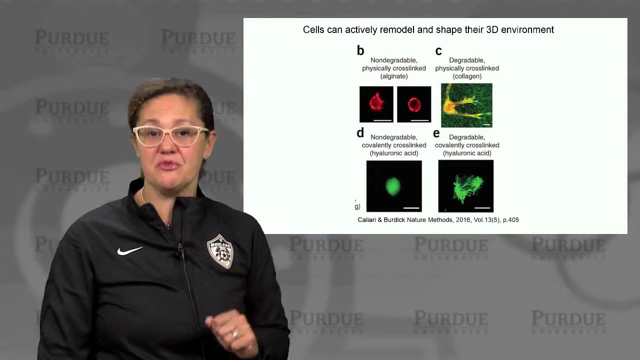 And they can be natural and native, such as collagen and laminin types that we would often see, mammalian cells, for example, surrounded in the body And in the body And in the body In natural organisms. okay, So cells can actively remodel and shape their 3D environment. 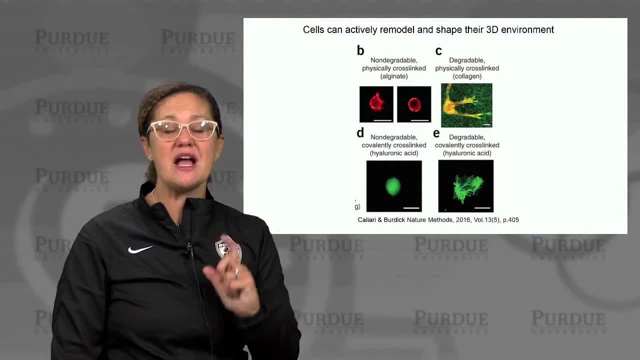 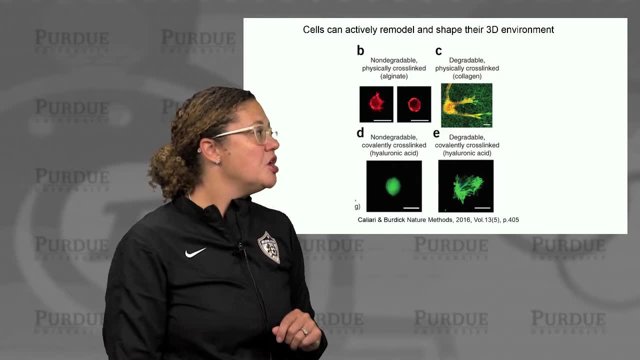 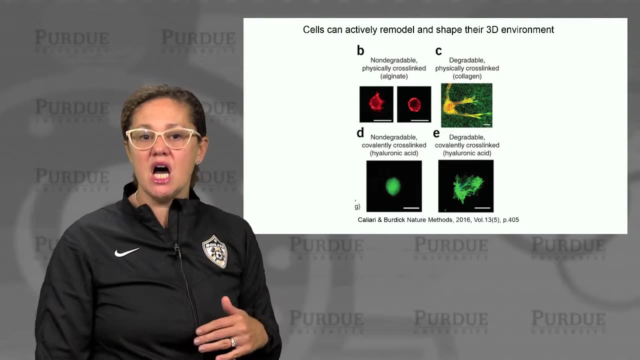 So again, this is that two-dimensional or, excuse me, two-directional communication between cells and the materials that they're surrounded in, And here's some examples. now we put in these different three-dimensional environments They can also not only being sort of natural or non-natural, or native, or 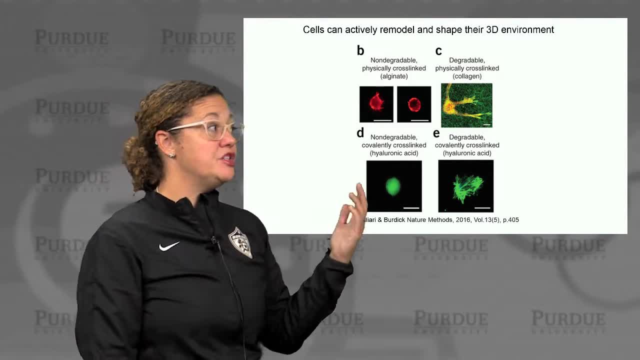 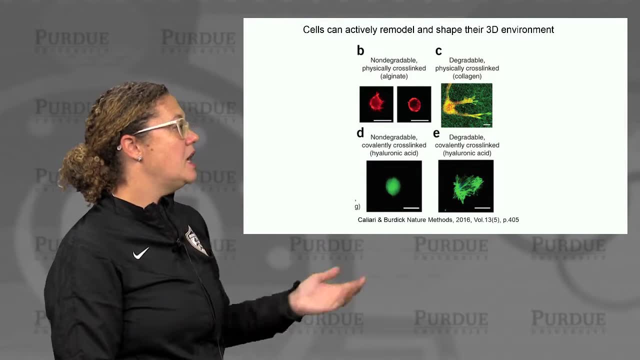 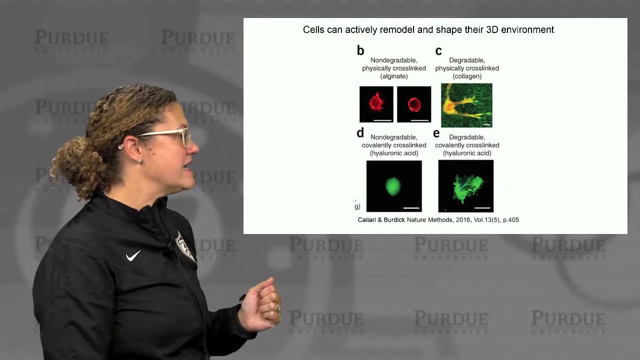 non-native. we can also have materials that are either degradable or non-degradable by the cells, And you can see that in the non-degradable materials, such as alginate or this artificially cross-linked hyaluronic acid, another natural component of many tissues, that in these cases, 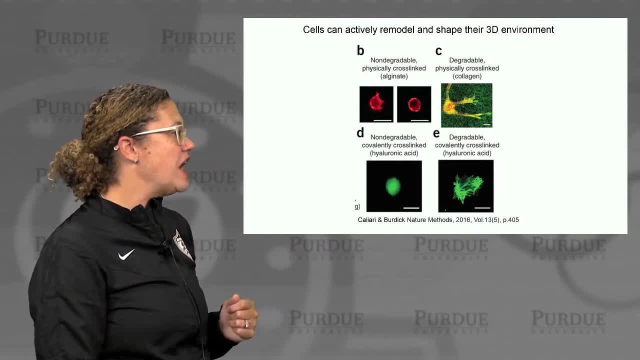 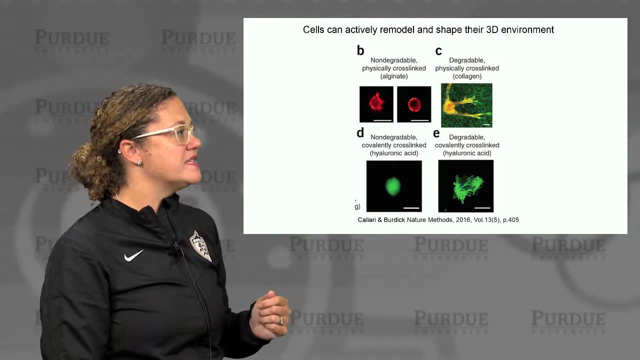 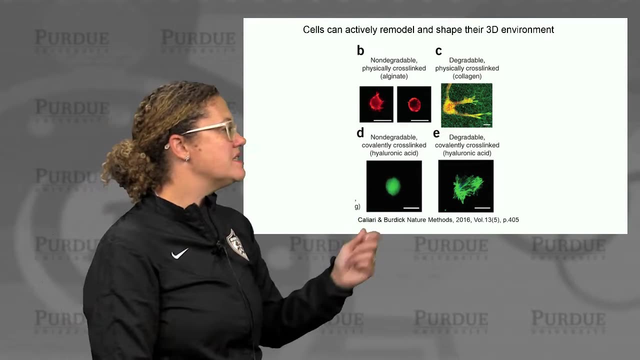 the cells are fairly confined right And their morphology is somewhat rounded, And you put the same cells in a degradable either collagen or, in this case now, a differently cross-linked hyaluronic acid, one that is degradable. you can see that the cells now are able to change their 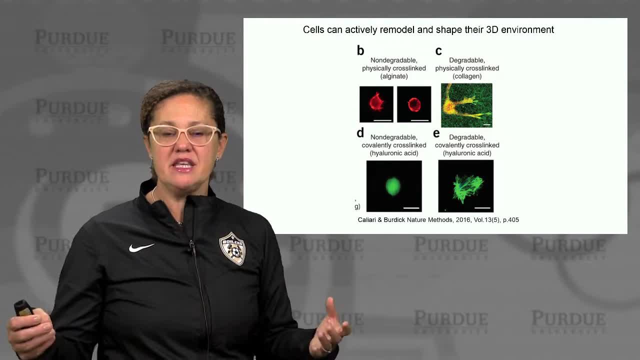 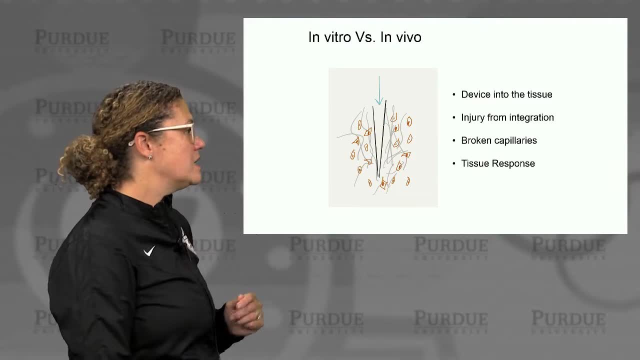 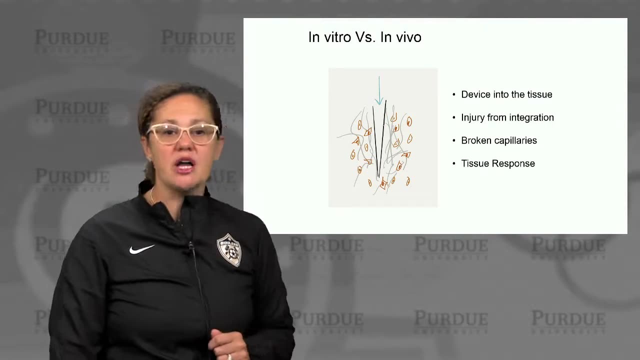 shape by degrading and manipulating the environment in which we put them in, And that's something that cells naturally do in their native environments. Okay, so we've mostly been talking about in vitro. We've talked about 2D and 3D, but let's also talk about in vitro. 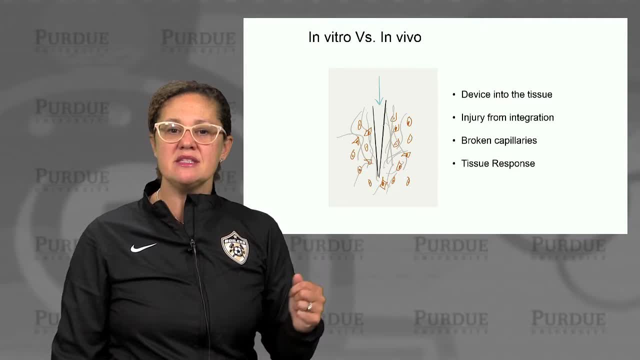 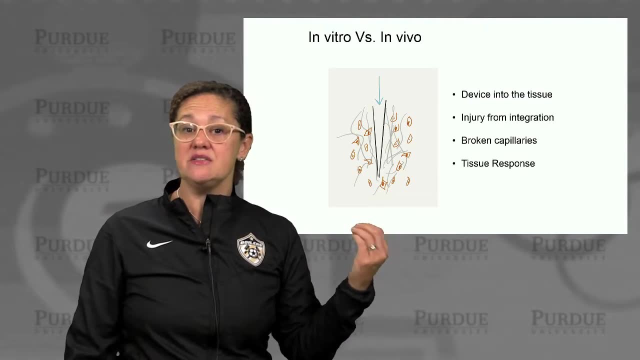 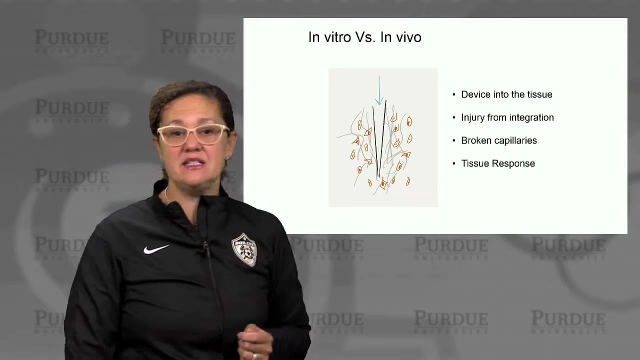 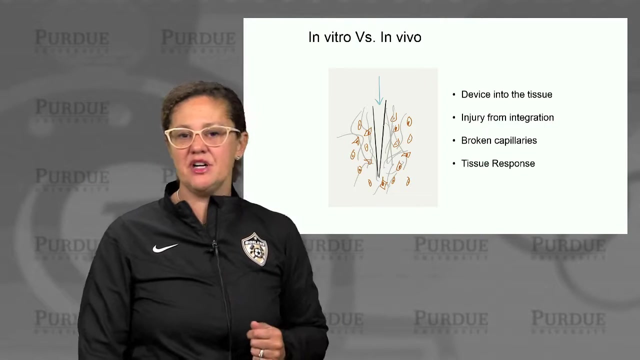 So in vitro we're typically putting the cells onto or into an environment, But in in vivo we're often integrating the device into the tissue And with that often comes injury from that integration, broken capillaries, other tissue damage and a little bit different of a tissue response. 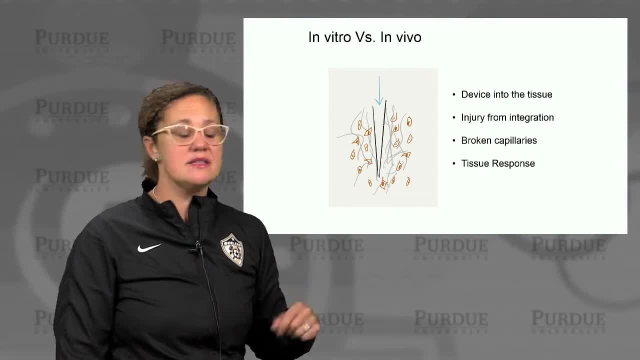 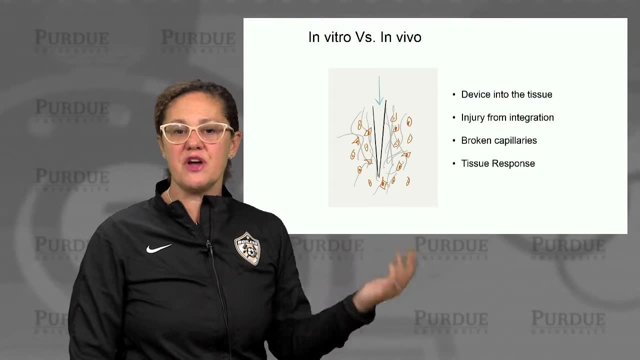 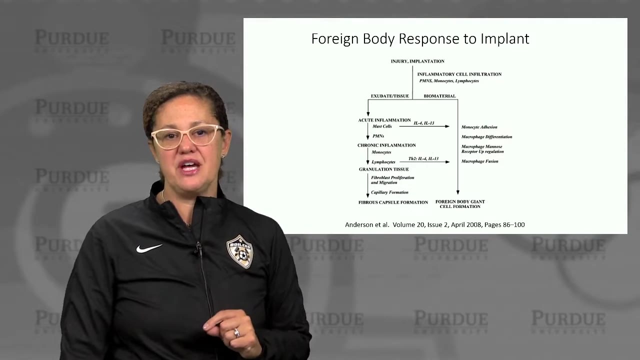 And so because of this acute injury in this more complex tissue response, because now if we're in a whole organism, we often have an immune system and other functioning components going on, And so this complicates our cell device biointerface. And so one of the things that typically happens when you put a large 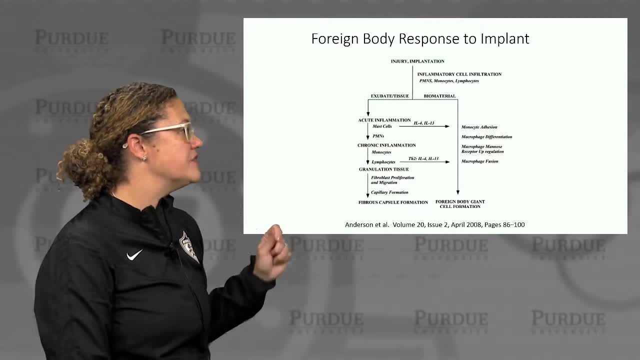 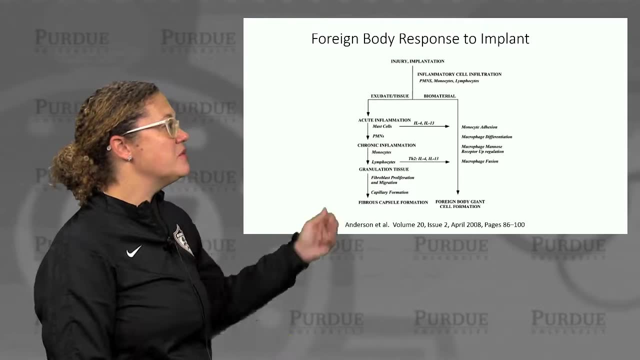 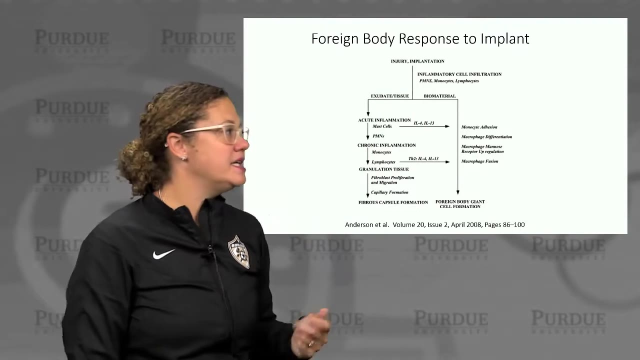 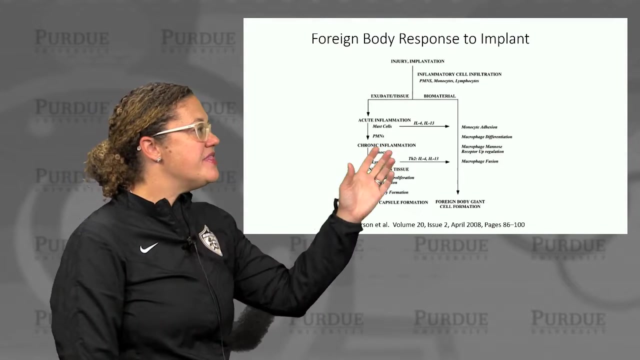 engineered device into the body is what's known as the foreign body response to the implant, And this happens over a course of time, beginning with an initial injury or implantation, And there's often initially protein adhesion and inflammatory cell infiltration from that injury. 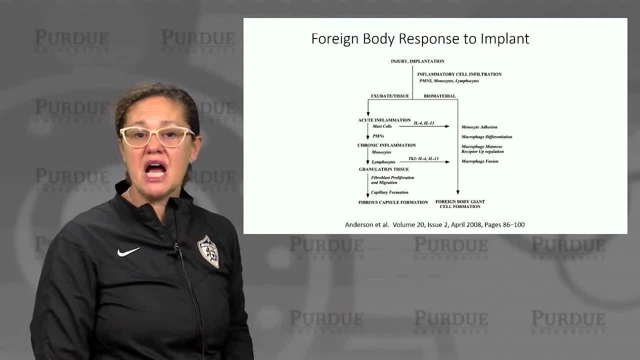 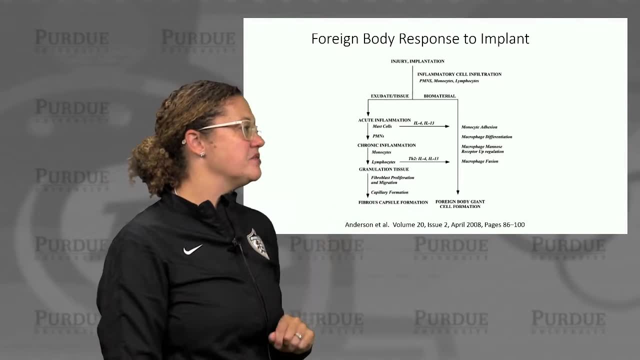 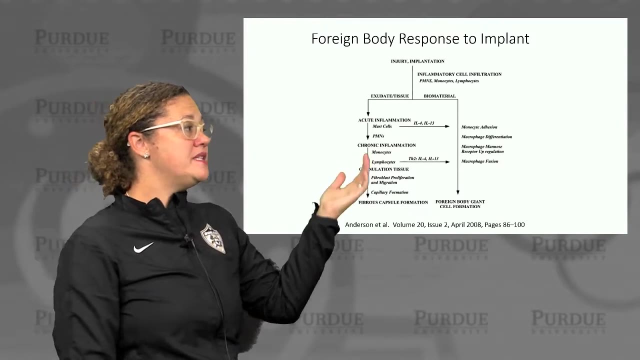 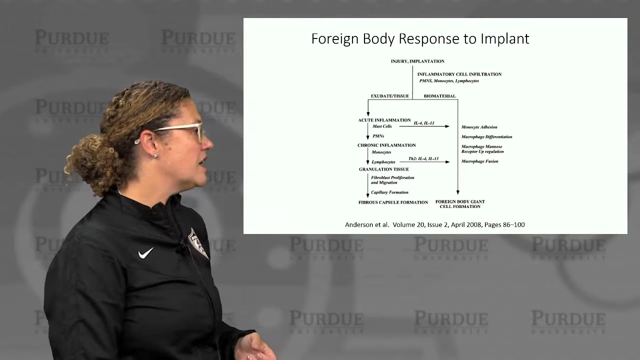 And then we have a continuation from an acute to a chronic affect, both at the material interface of our device and within the surrounding tissue, And again this propagates from an acute inflammation into potentially chronic inflammation and ultimately an encapsulation of our device with fibrous tissue. 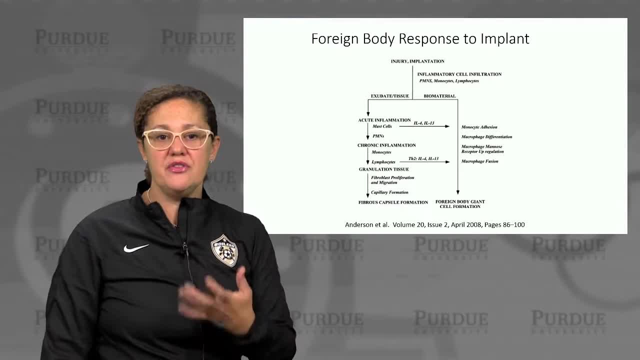 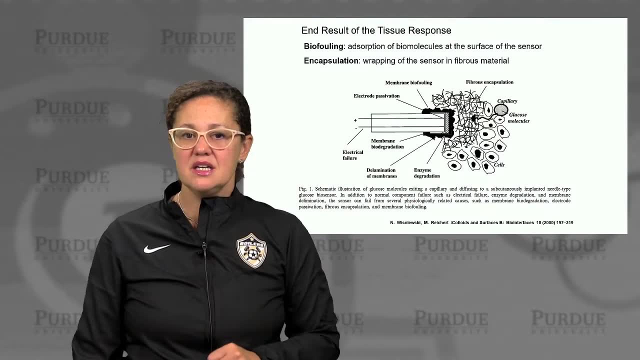 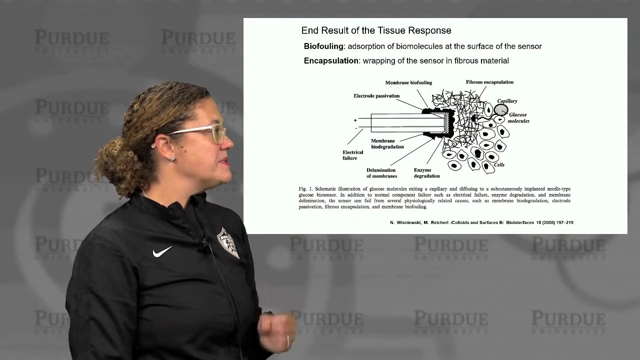 Obviously something that we often don't want if we want a good, healthy integration of our cells and tissue and our device, And so the end result of a device being put into the body is often this sort of encapsulation and fouling due to this fibrous capsule that's formed around here. 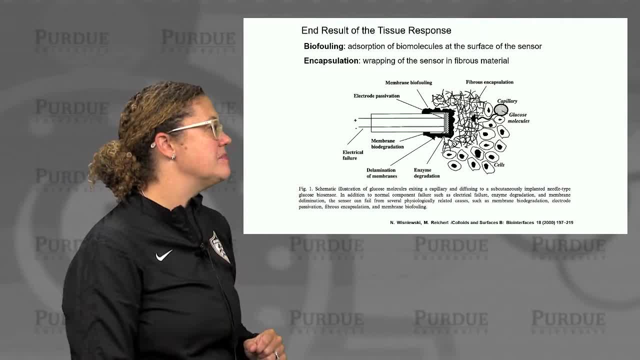 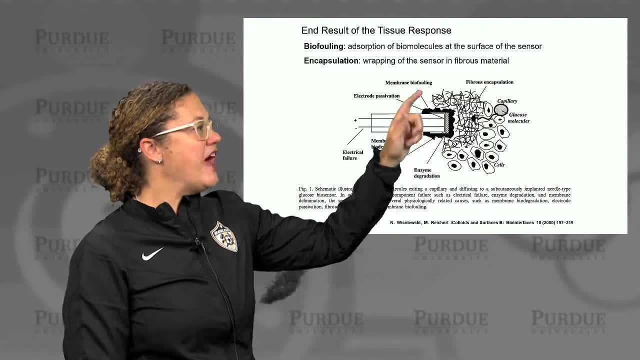 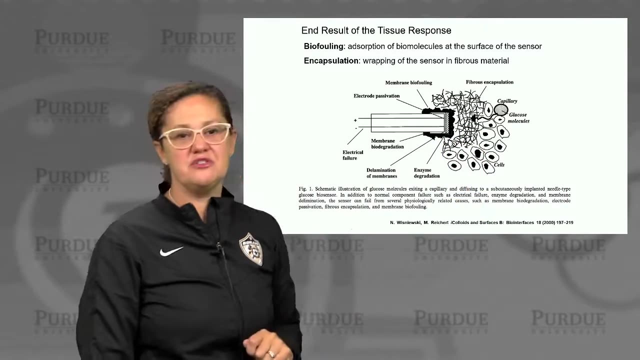 We have an image of a sensor that's been placed into the body and around the sensor membrane and the sensor components. We have protein adhesion and fouling of that device, as well as a fibrous encapsulation. This sort of forces away the cells of interest, the natural cells and the capillaries. 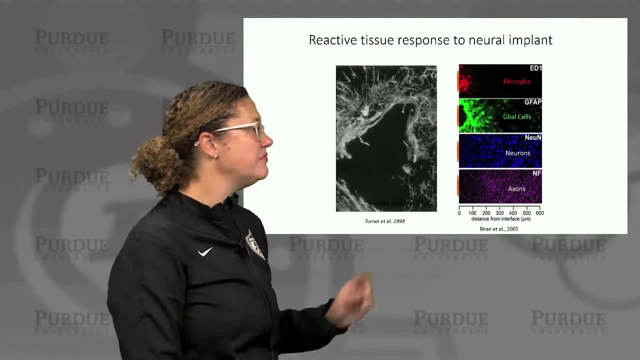 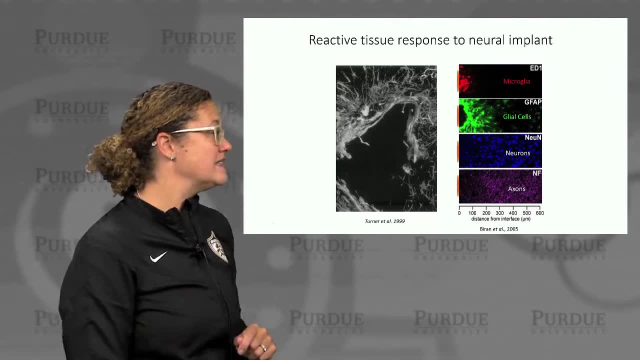 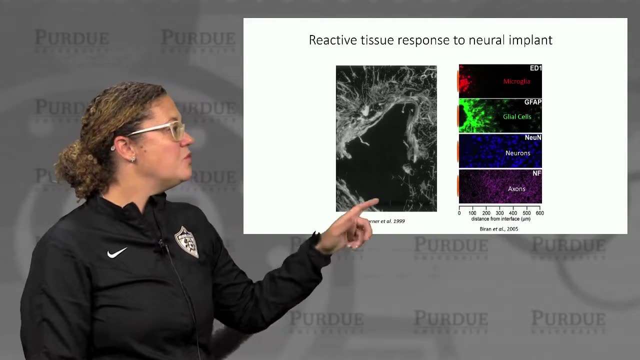 and typically the systems that we want to interface in. So here's what this can look like in the brain. Here's a reactive tissue response to a neural implant. So in our last lecture we were talking about the brain computer interface and neural implants as a type of bio-hybrid device. 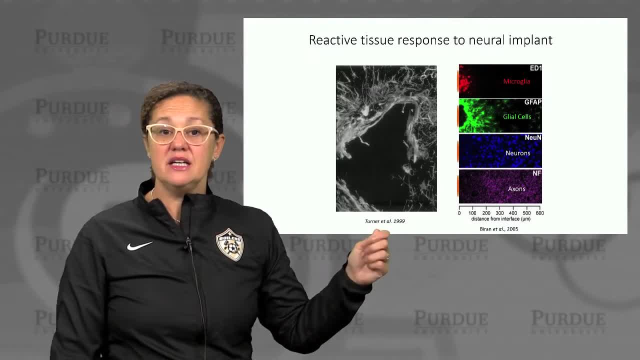 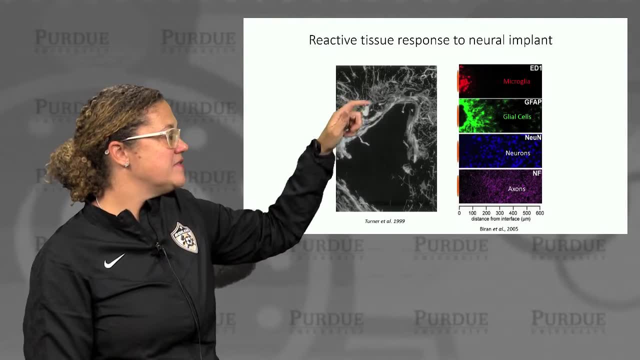 And what you see here is a very typical after that. in this case, an electrode was removed from the brain And we can see the site where the electrode was And you can see all this fibrous tissue and what's called a glial scar. 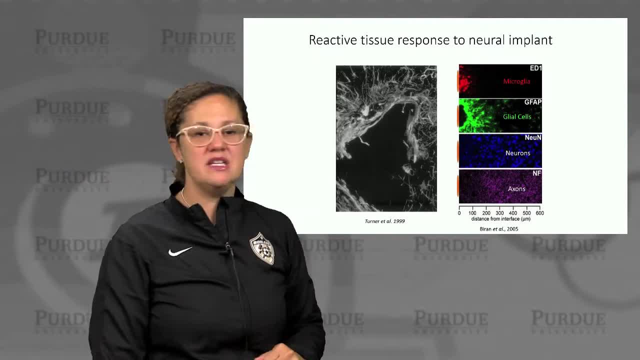 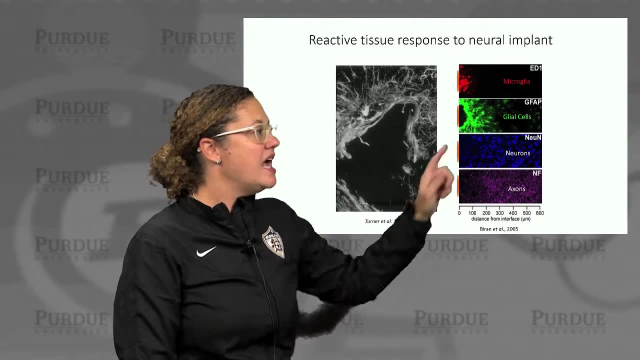 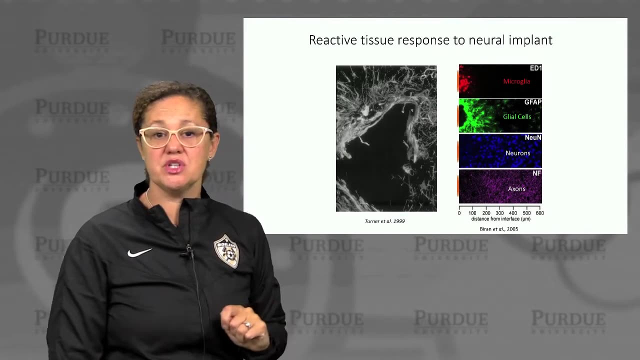 So this scarring around. And so now, if you look at some of the individual cell components, we can see the resident immune cells of the brain, the microglia And the other glial cells which are reactive and have been activated to form this glial scar around the cells. 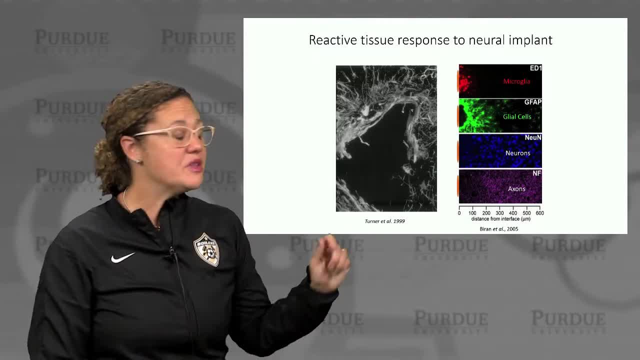 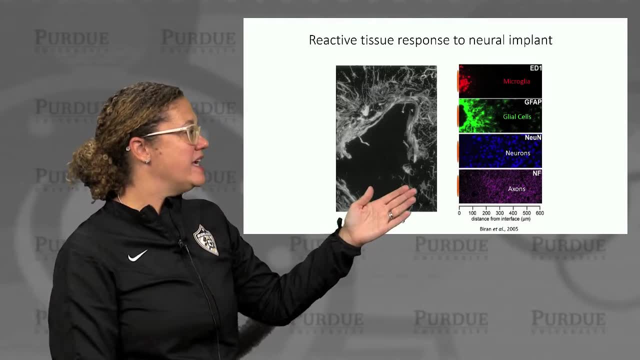 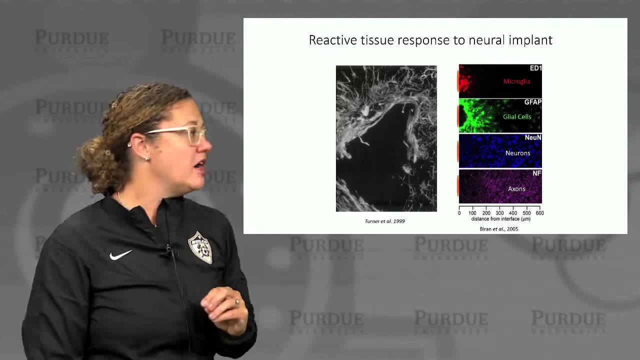 And now most often the cells we're interested in interfacing with. for the brain computer interface, the neurons and its axons, you can see, have now been pushed away and are no longer near the electrode surface that's depicted here. So this is obviously something we don't want quite often when we're making our 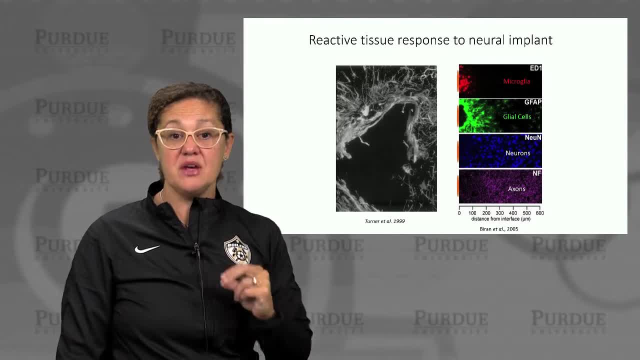 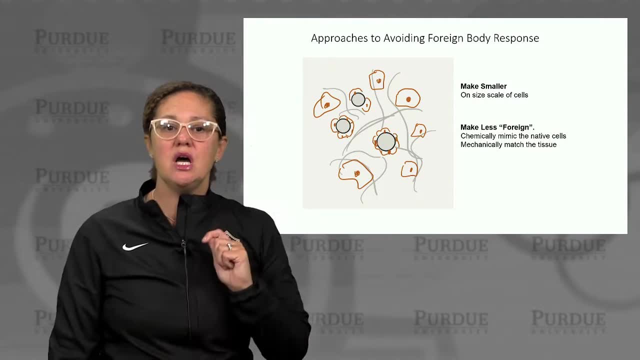 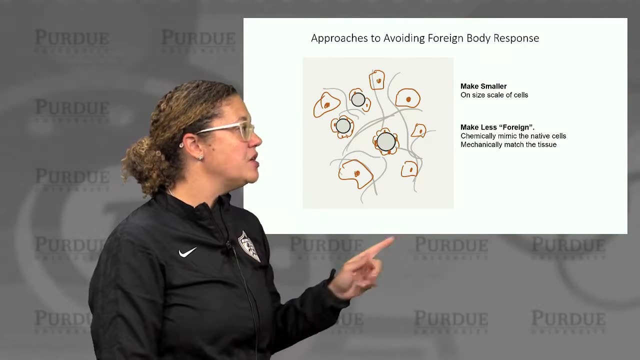 bio-hybrid devices. We want a healthy integration of cells and tissues with our engineered components. So there are, I think, probably the two winning and probably most promising approaches to avoiding The foreign body. response is kind of two-fold, And one is to make our devices smaller.